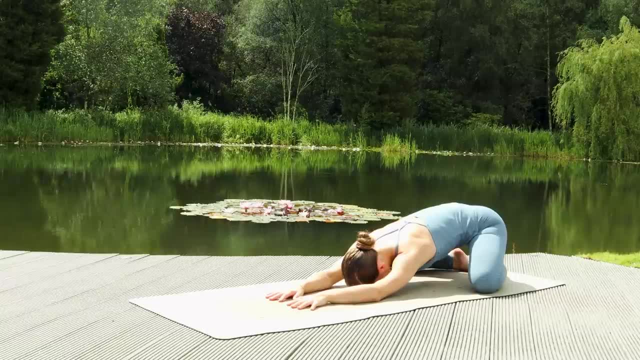 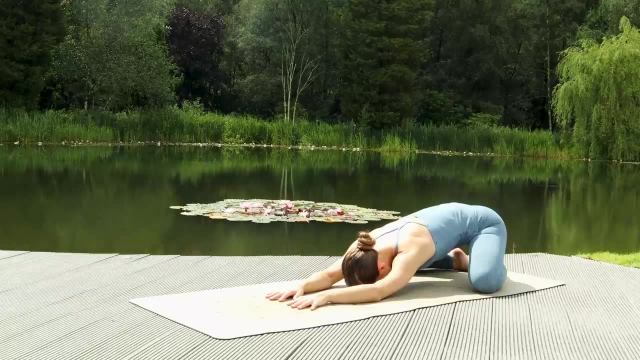 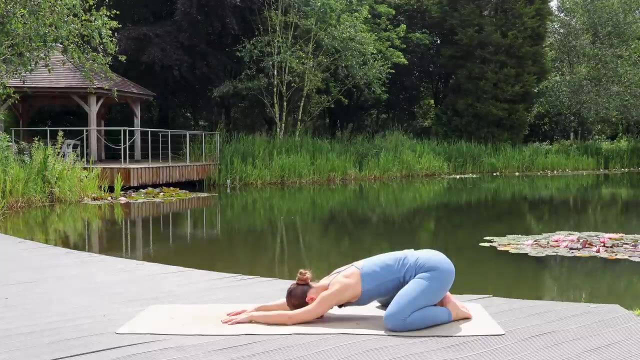 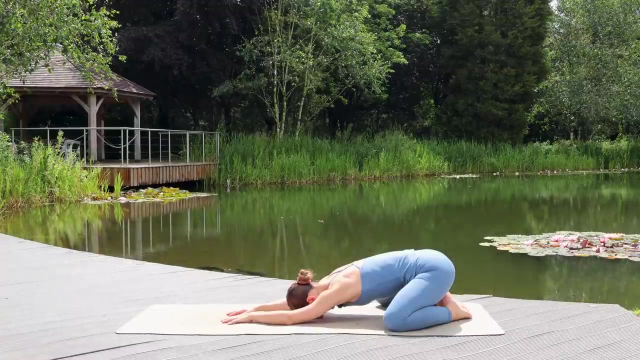 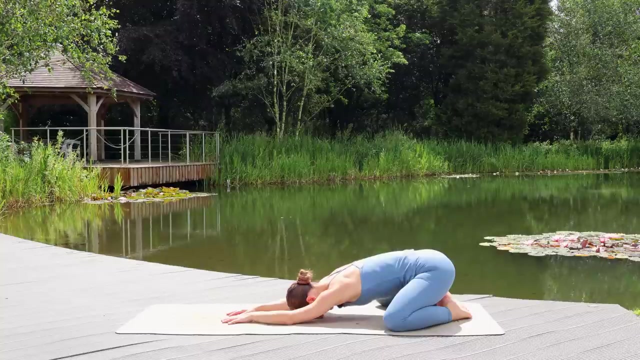 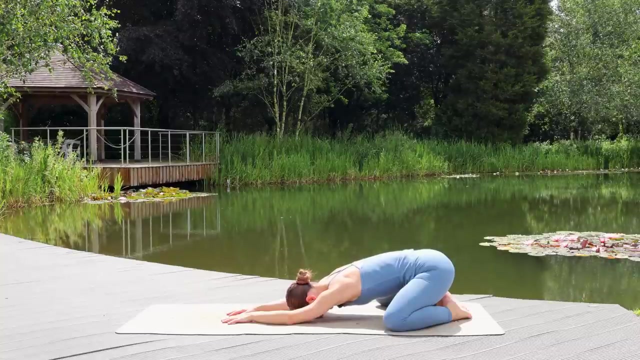 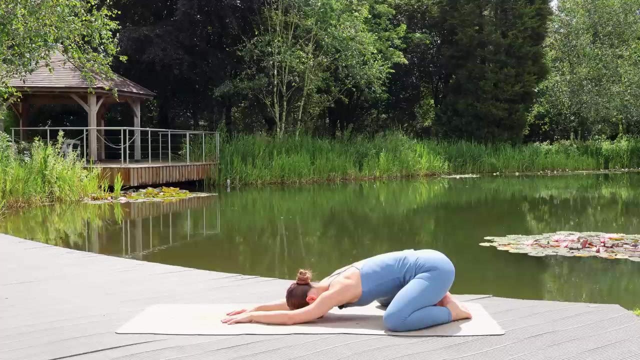 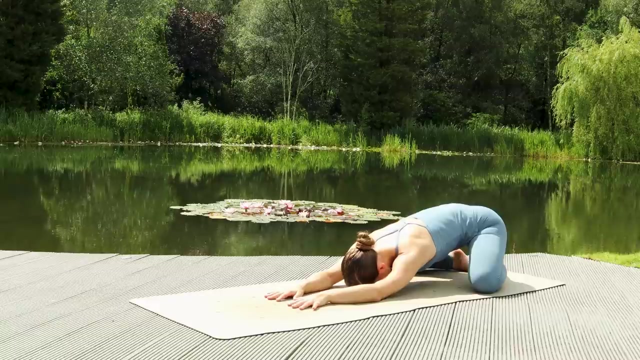 few moments in stillness here so you have chance to pause, to reconnect with your body and your breath, Bring your awareness to your inhale and your exhale, finding a steady breath and, at the same time, relaxing your body. Staying in child's pose. walk your hands over to the left side of your mat and place. 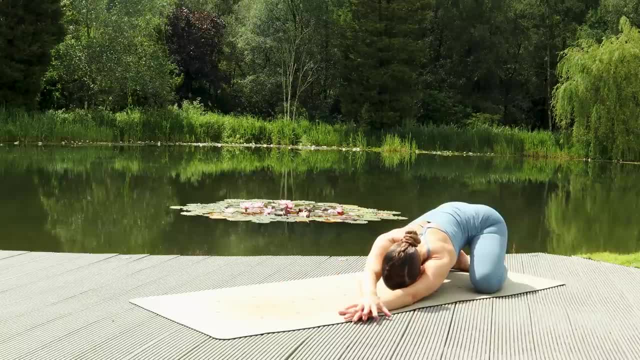 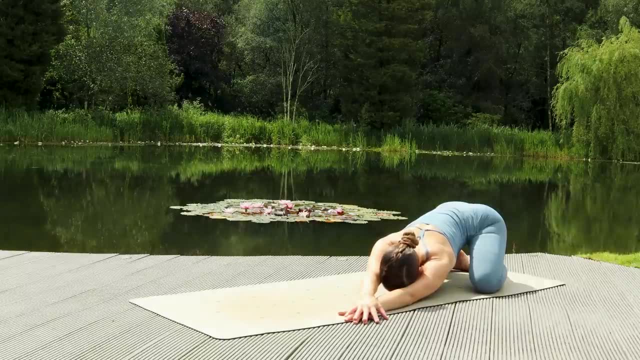 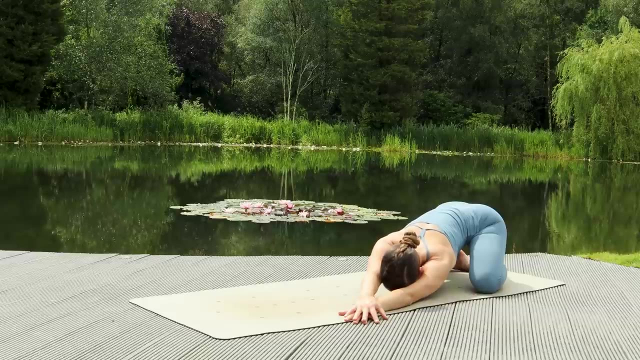 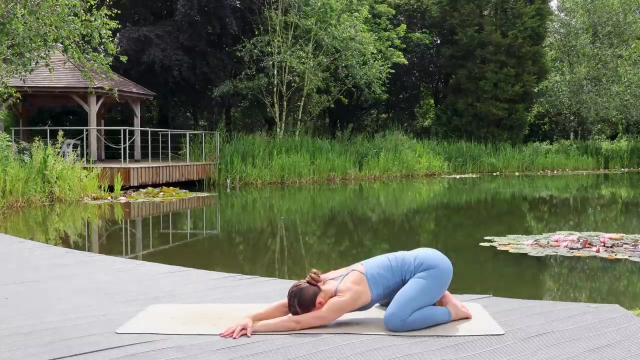 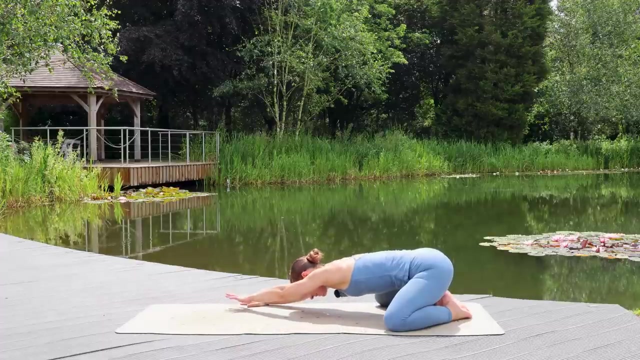 your right hand on top of your left And you're looking to feel a slight stretch down the right side of the torso and along the arm And walking the hands over to the right side of the mat. this time the left hand will stack on top of the right And you're looking to feel a stretch down the left side of the. 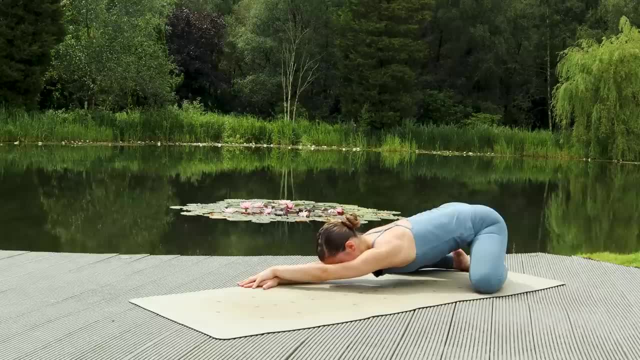 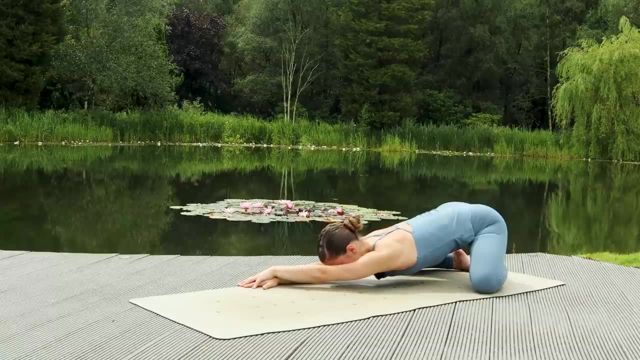 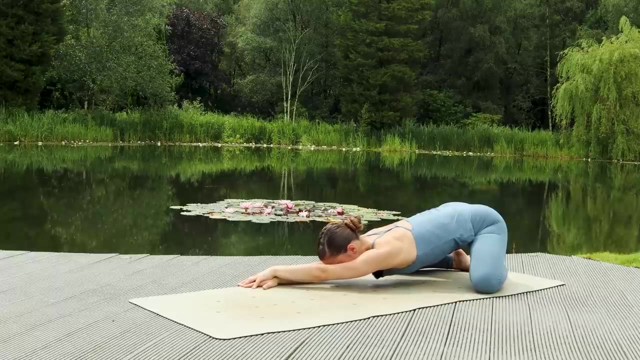 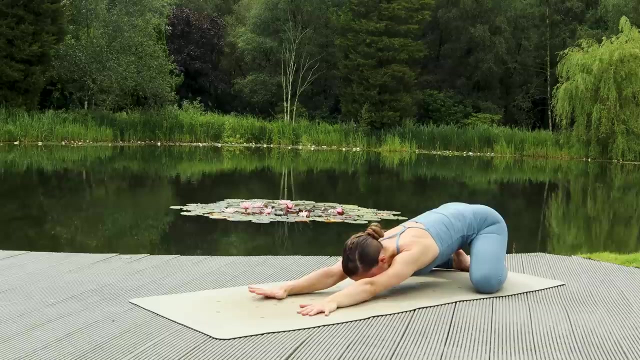 body And the right hand will press against the left side of your mat And, walking the hands back in towards the middle, Reach your hands as far forwards as you can so you find that sense of lengthening all the way down your back. 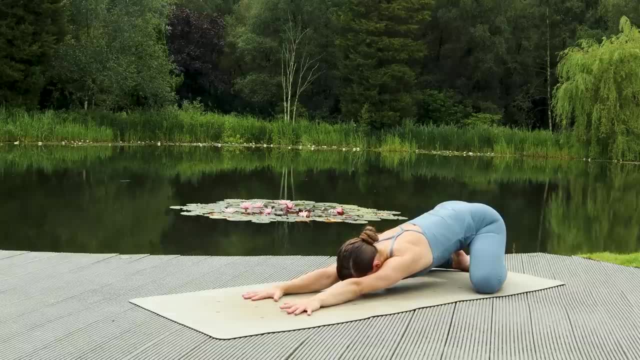 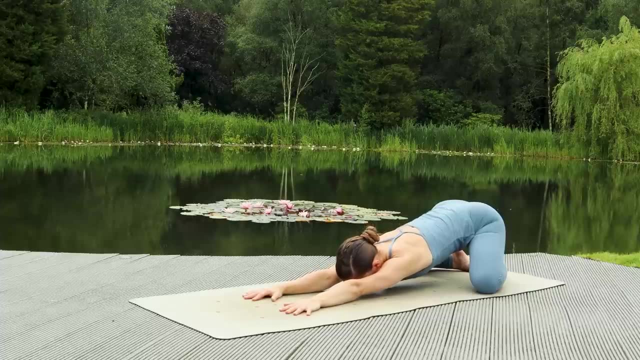 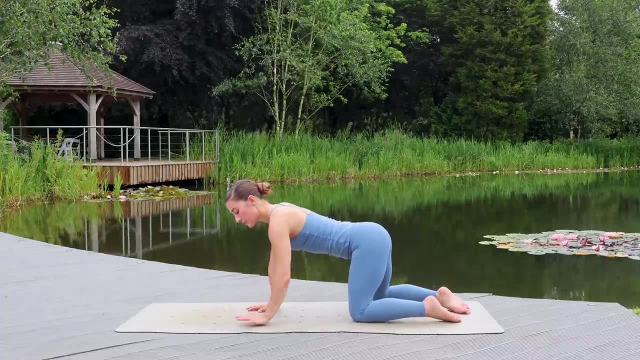 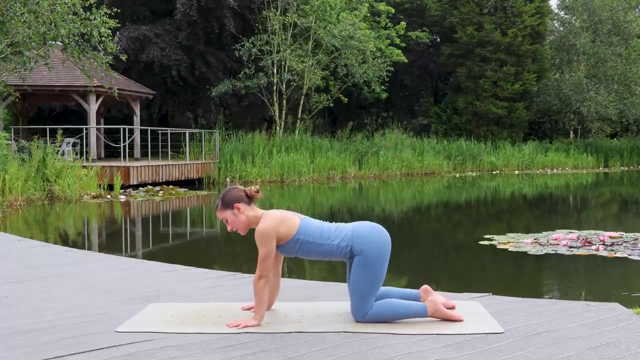 We'll take a full breath in here through this nose and exhale through your mouth. Come up onto your hands and knees- so tabletop position- and you're looking to place your hands under your shoulders and your knees under your hips. We'll start by rocking over to the left and over to the 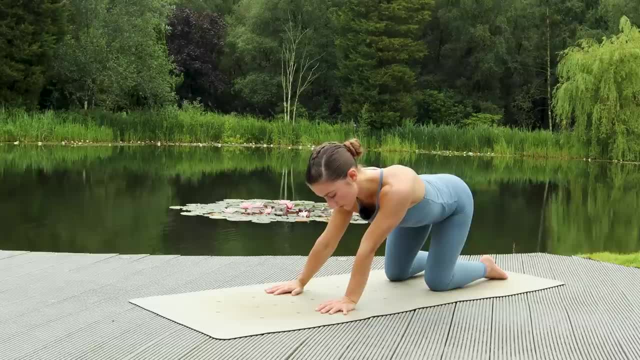 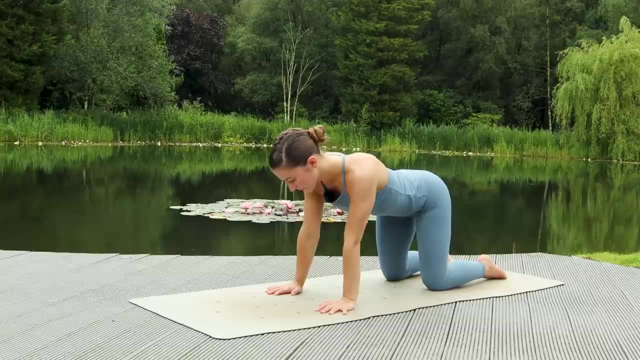 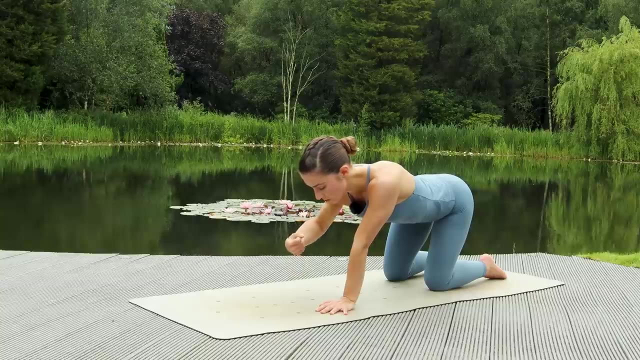 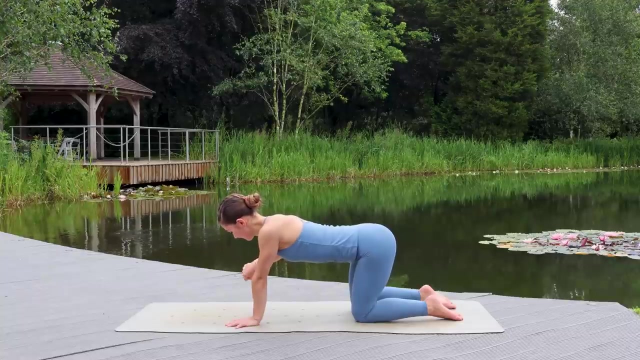 right. So you're shifting your weight to each side of the mat to begin warming up the wrists. The next time you lean over to the left, make a fist with your right hand and start to roll out your wrist, And then we'll switch, So planting the right hand. 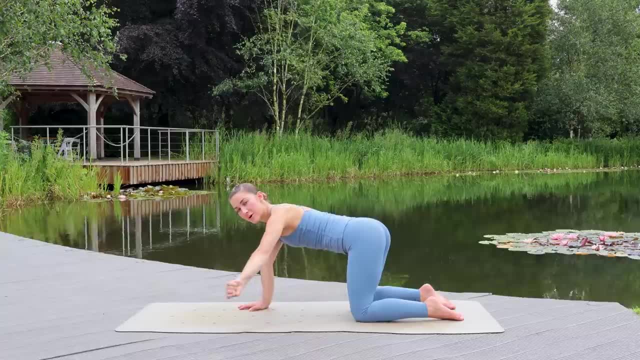 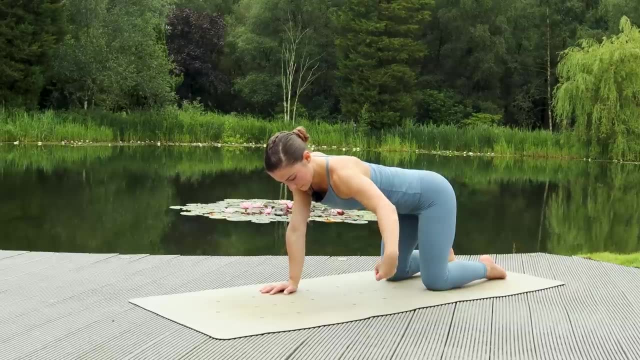 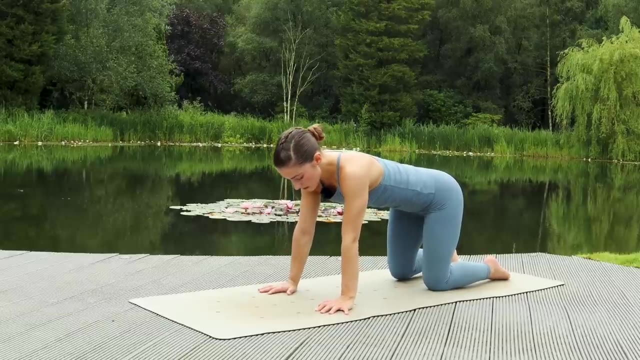 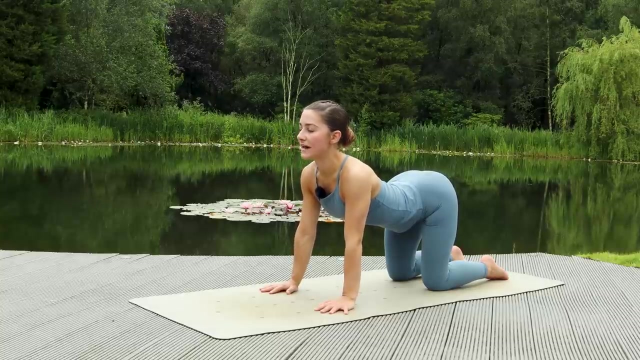 shifting the weight into the right hand and rolling out the left wrist And planting the left hand back down With an inhale. lower your belly to begin arching your spine and gaze forwards As you exhale. push the floor away round your back and bring your chin to your chest. 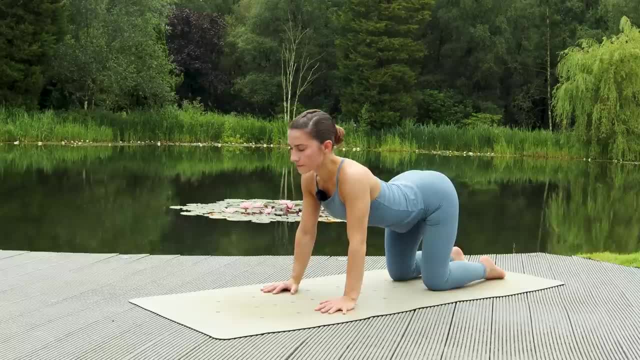 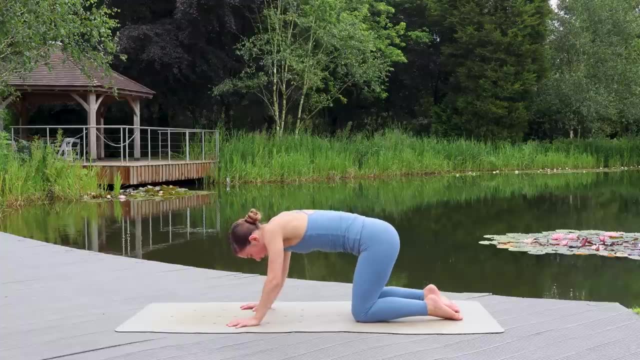 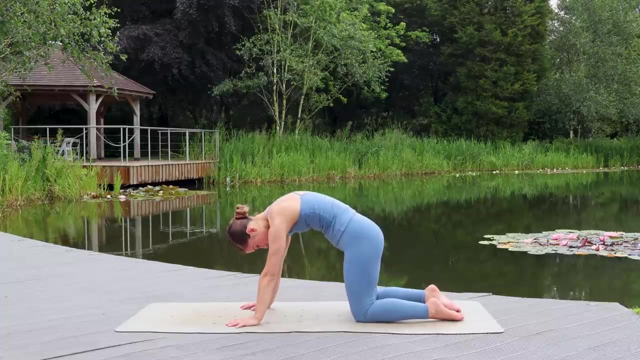 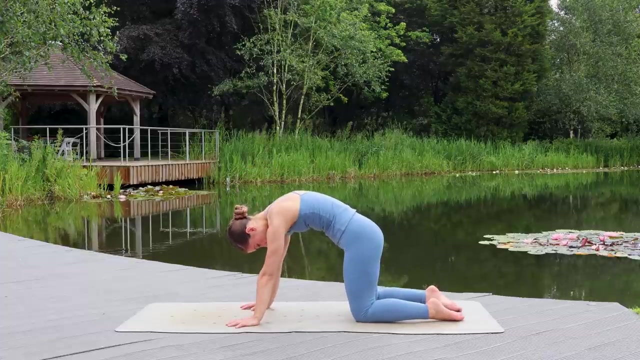 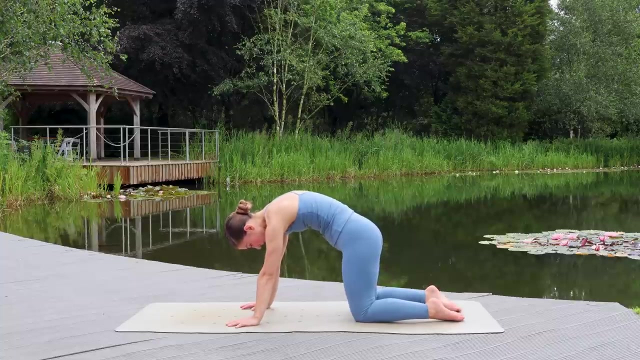 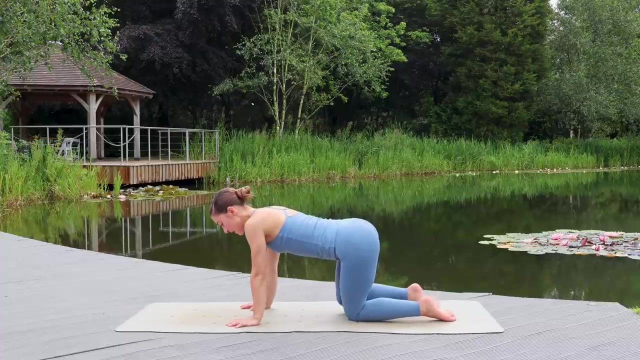 Inhale as you arch the spine, Exhale as you round. Keep this flowing with your breath. One more inhale and exhale, Then finding a neutral spine, a relatively flat back position. extend the right leg- you can keep the toes on the mat for now and reach your left arm forwards, keeping 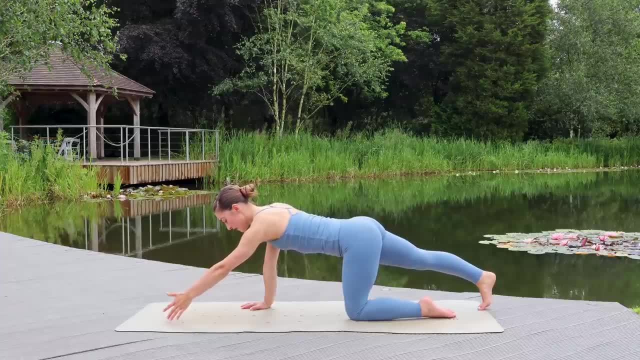 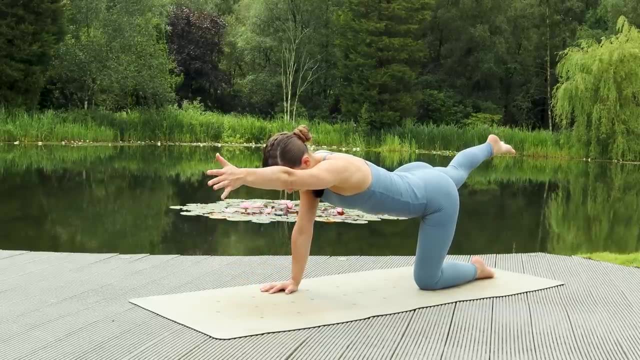 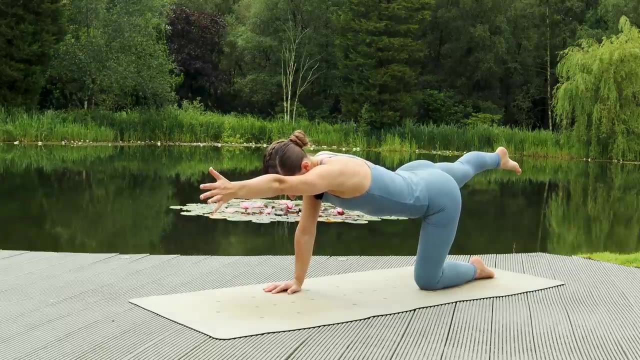 the fingertips on the mat for balance And when you feel steady, start by lifting the leg and if you feel ready, lift the arm also. So you're coming into this balance, reaching the left fingertips forwards, the right toe tips back. 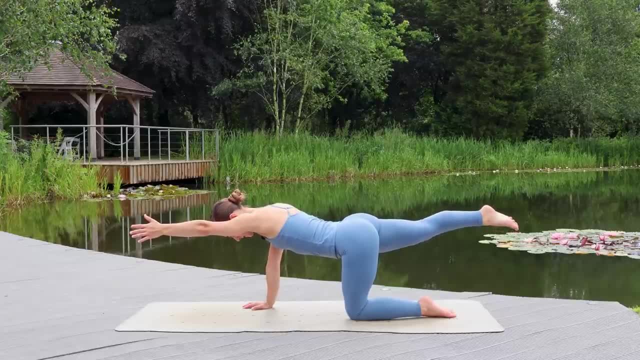 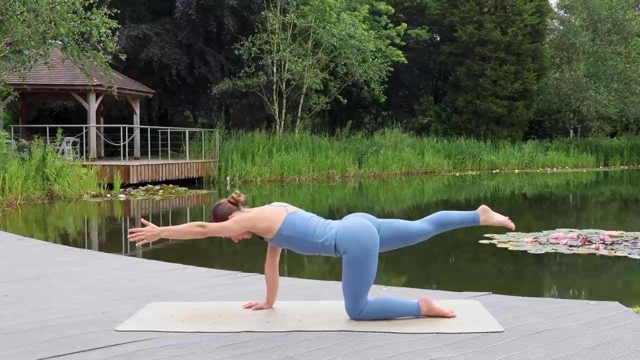 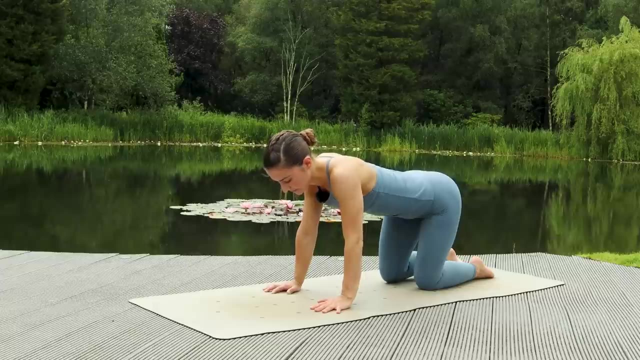 If you're feeling any tension in your neck, bring your chin to your chest, Hold for an inhale, exhale and release, bringing the hand and the knee back down, Finding the left leg. now toes stay on the mat. reach the right arm forwards, keeping. 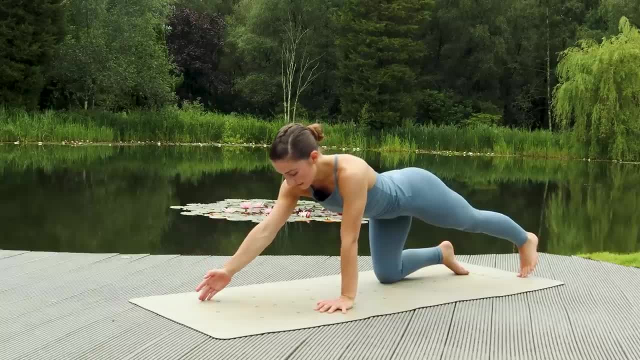 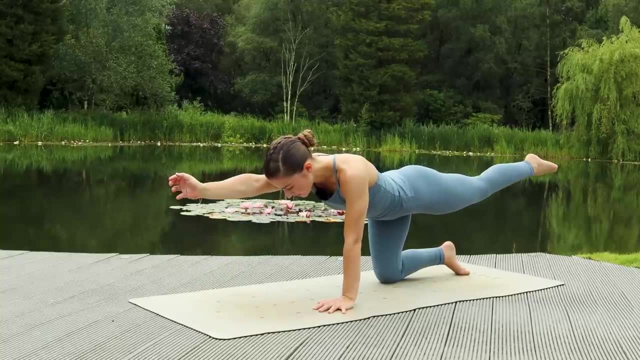 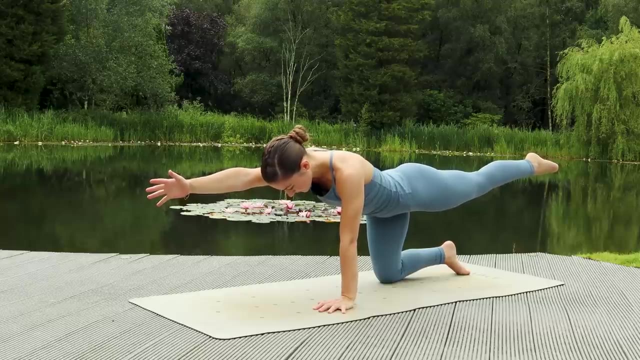 the fingers on the mat for now And, to begin, lift the leg and if you're feeling steady, you could also lift the arm. So you're reaching the arm and the leg away from one another to create one long line as we hold this here. 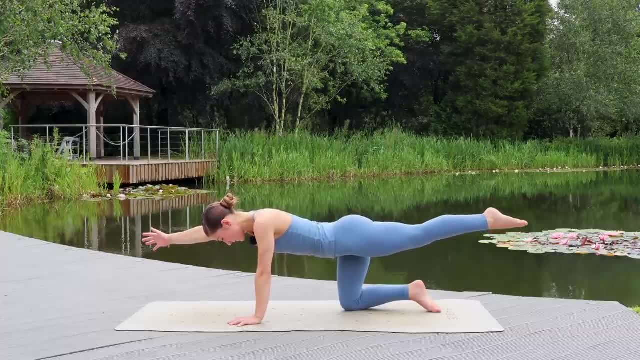 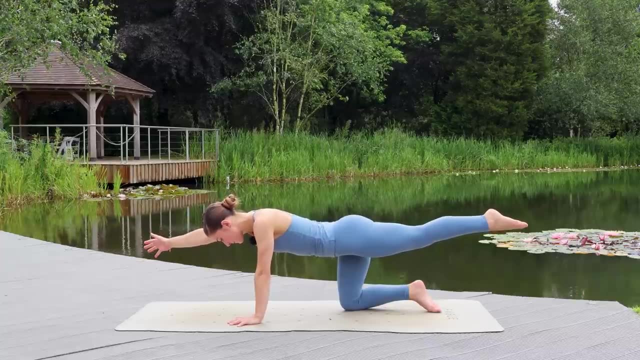 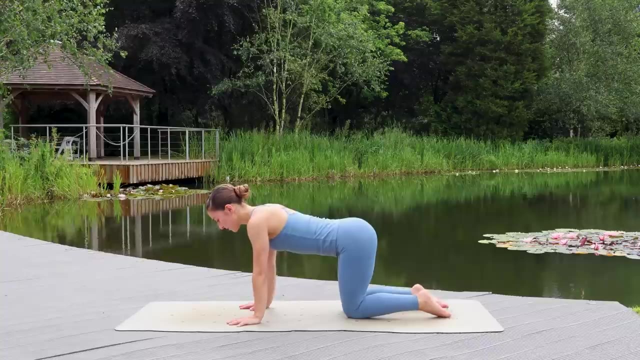 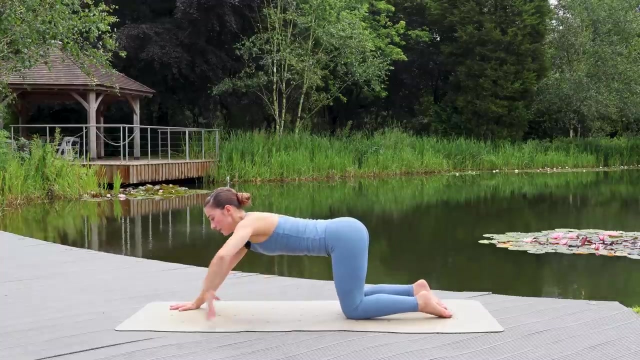 Take the tension out of the neck. relax, chin towards the chest Exhale Hold for an inhale exhale release. bring the hand and the knee back to the mat. Good work. Then, keeping your hips directly over your knees, walk your hands forwards and slowly. 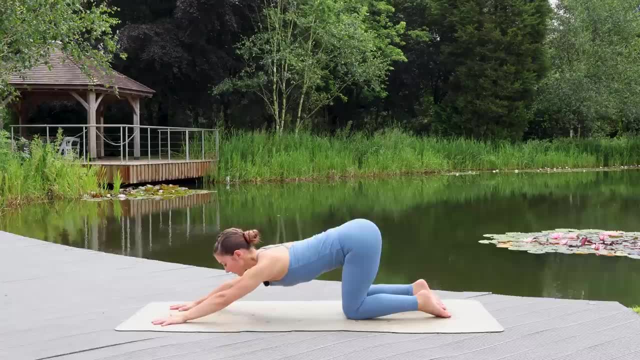 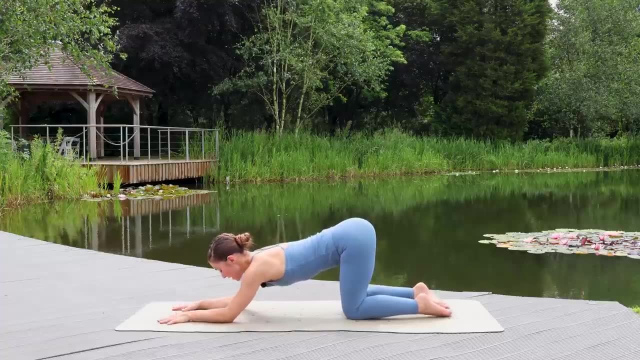 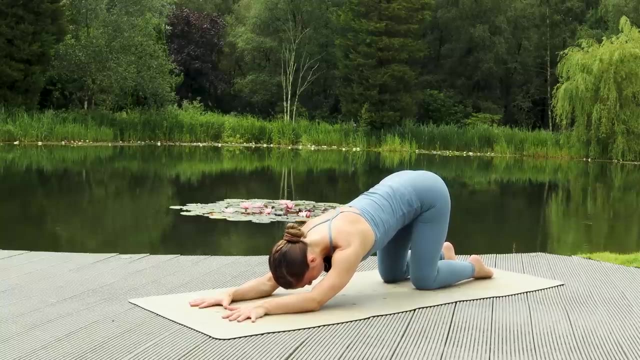 let your chest start to sink down. This may feel quite extreme, so you could bend your arms so that your forearms come down to the mat And relax your chin in towards your chest. so you're looking to feel a little opening through the chest. 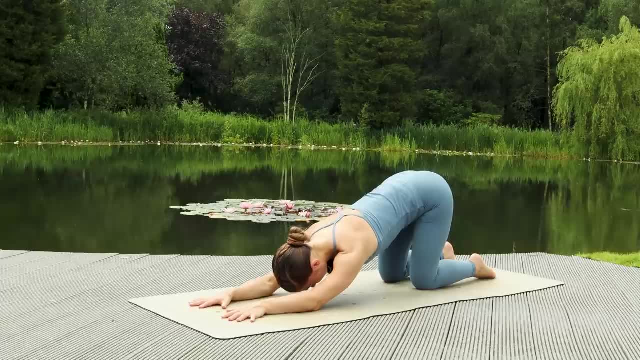 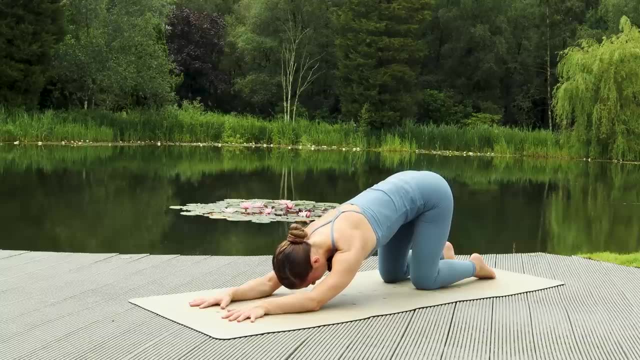 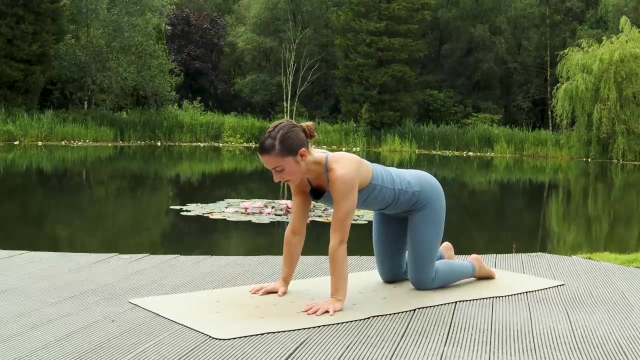 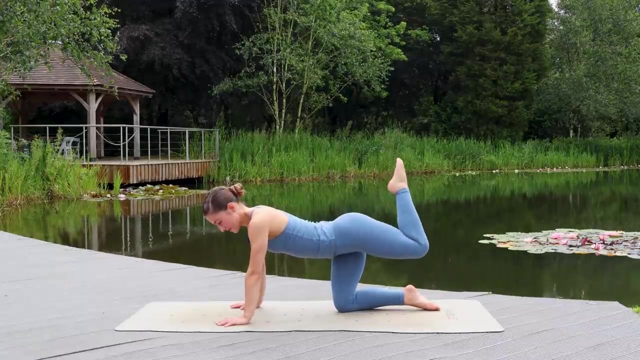 You may even feel some intensity in the upper back. Inhale in position, exhale it out. Then come back to your hands and your knees. Open the left knee out to the side and start to draw circles with the leg so you can circle. 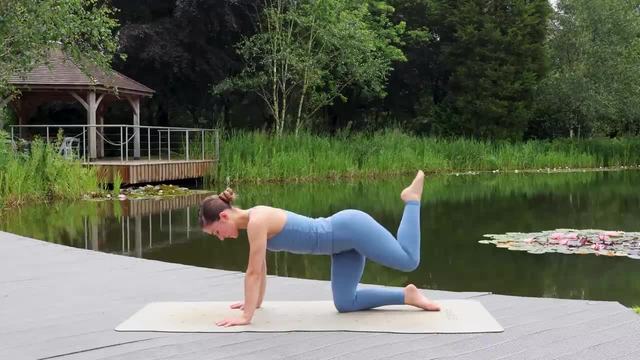 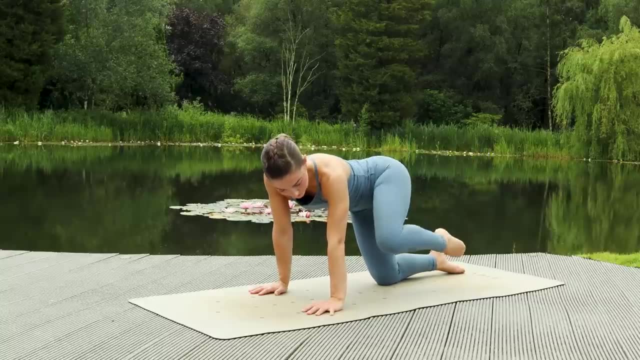 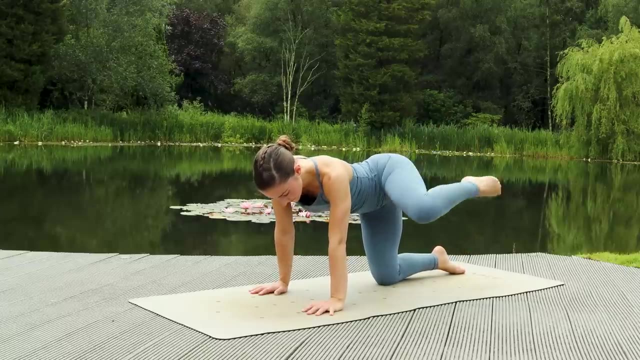 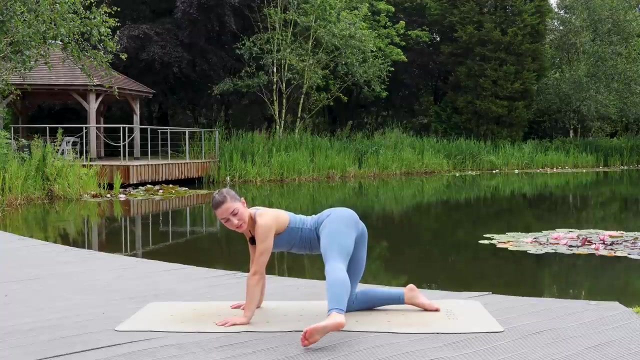 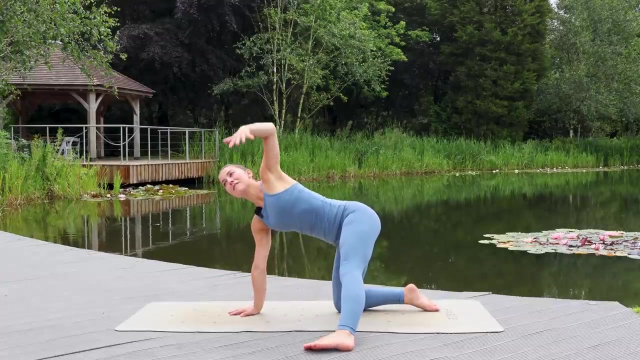 the leg away from you a few times And then reverse and circle the leg in towards you a few times. Good, The next time you lift the knee out to the side, extend the leg and lower the foot, Then bring the right hand towards the middle of your mat and reach the left arm up. so 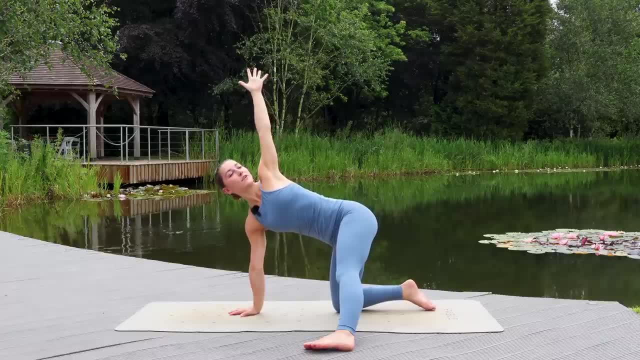 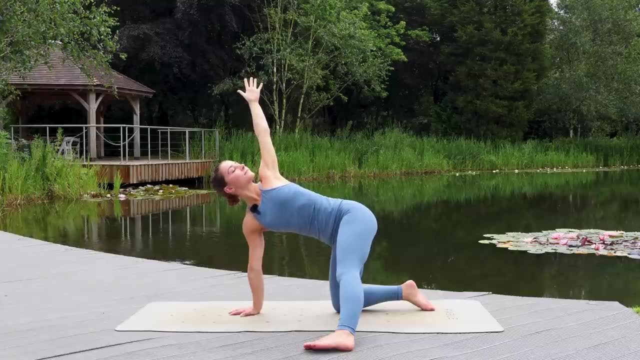 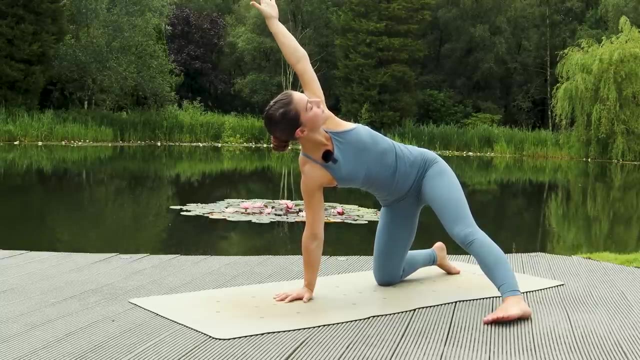 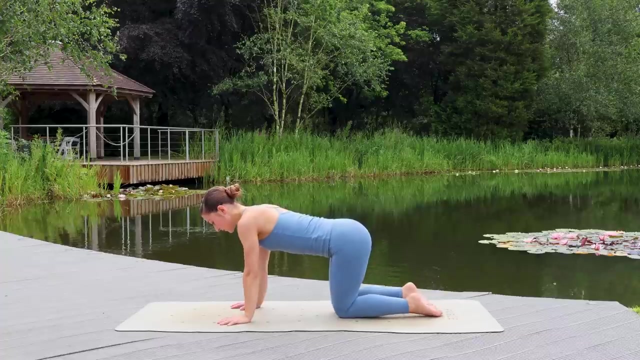 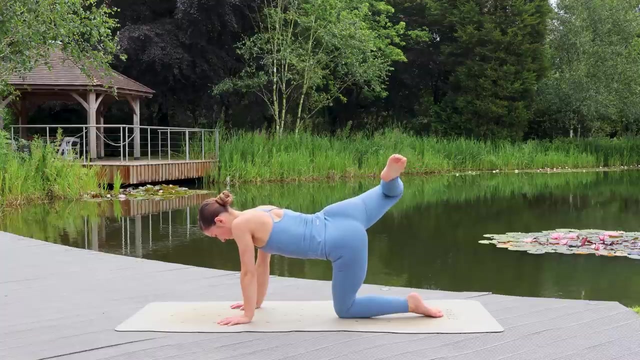 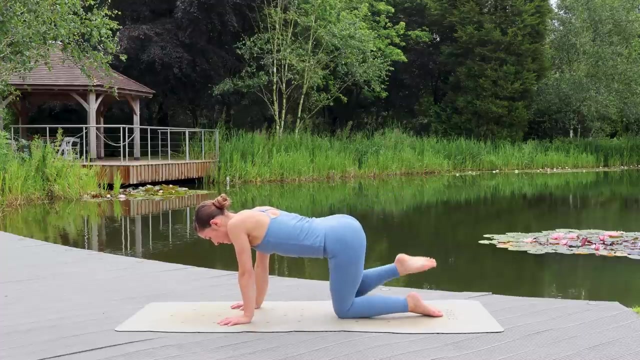 twisting open. If it feels okay for your head and your neck, you can gaze up towards the sky. Come back into Tabletop Hands and Knees position and start to circle the right leg away from you a few times And then towards you a few times. 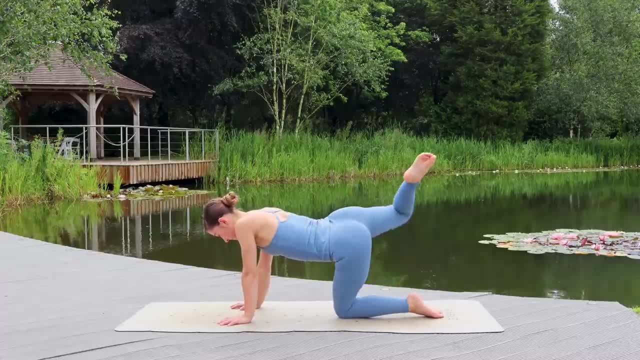 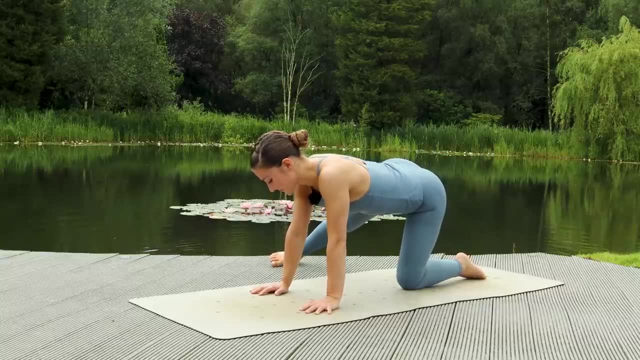 Good, Good, Good, Good, Good. If you feel you want to press your crossed hairs, Choose this position. When you bend the pistol pushing towards you, you pull the right arrow to your left hip, And this here is good Good. 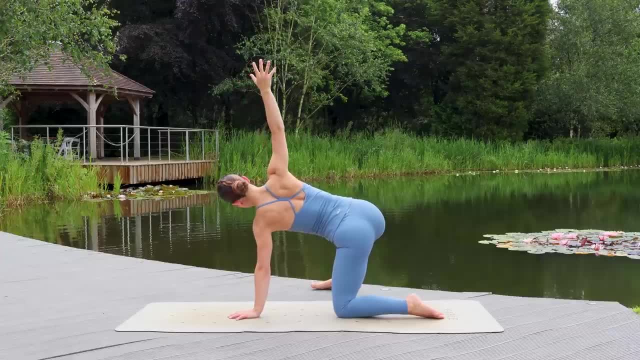 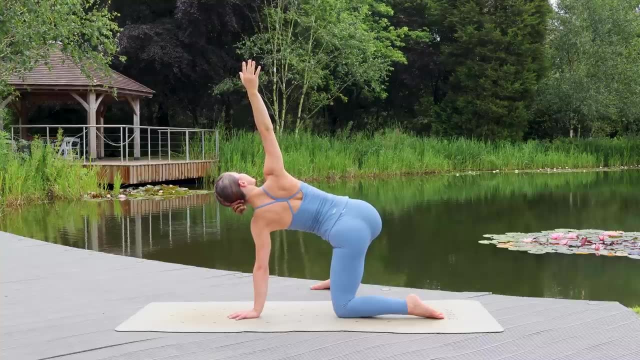 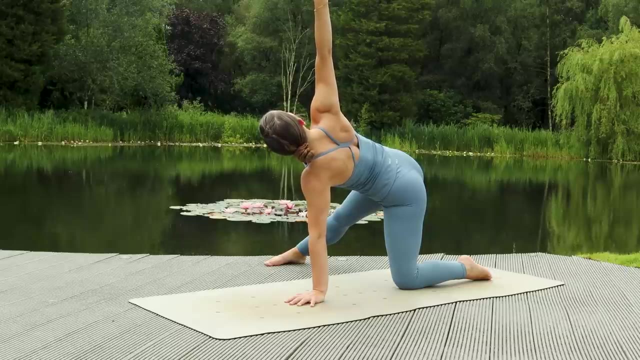 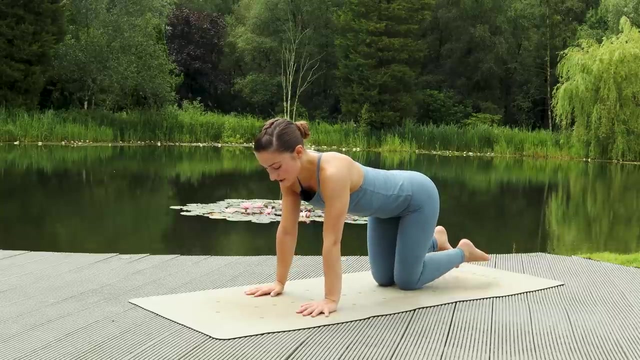 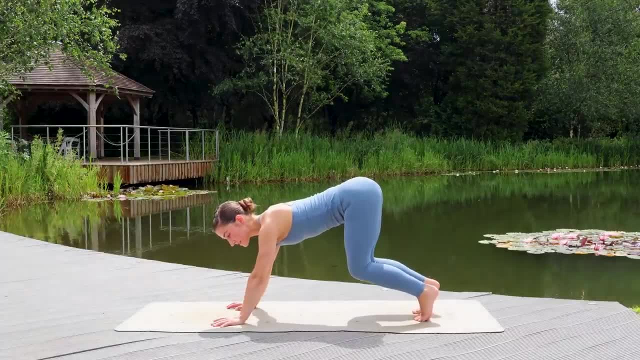 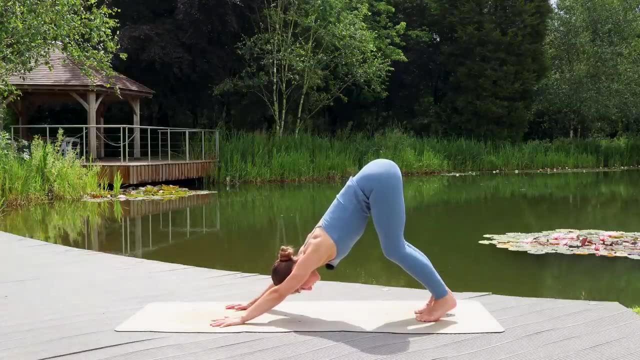 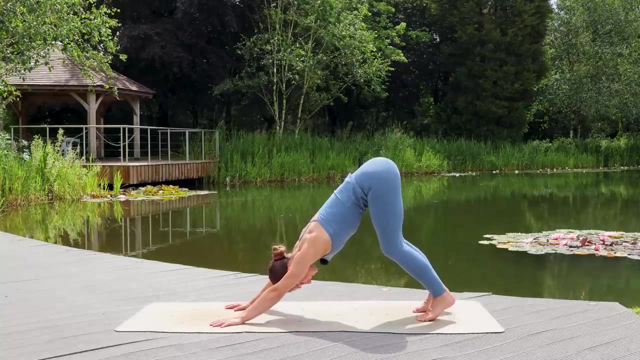 Then begin to lift the hips up. you can keep a bend in the legs as you push your weight back towards your feet. We're coming into this upside down triangle downward dog position. When you arrive here, keep your chin relaxed in towards your chest. focus on pressing through. 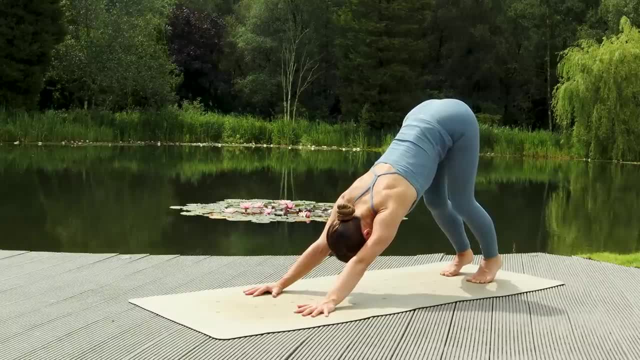 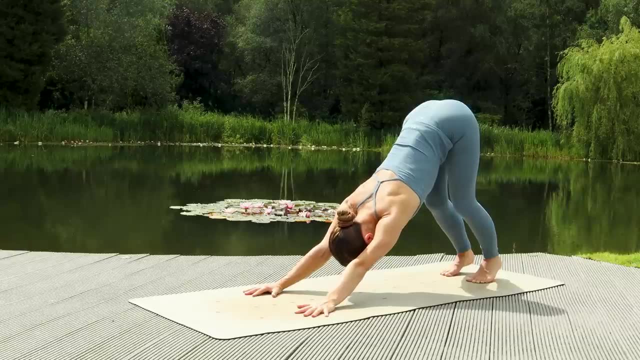 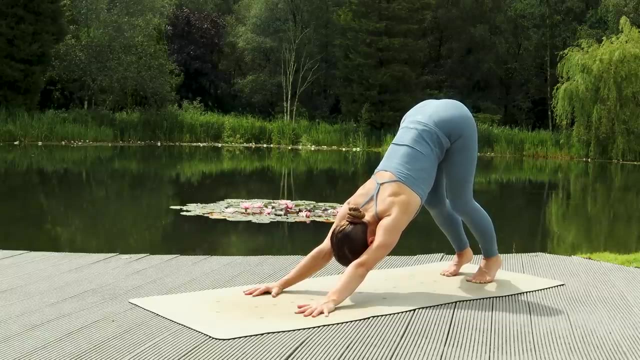 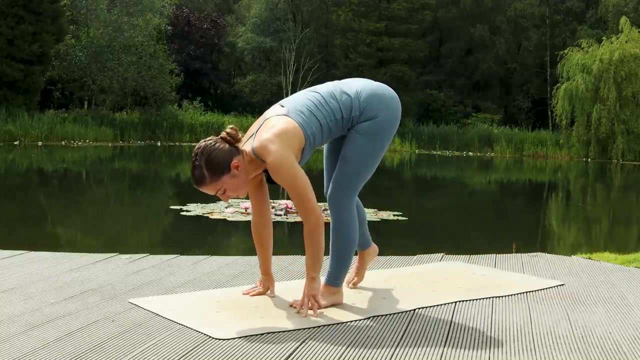 your hands and your feet. Don't worry about grounding the heels, don't worry about straightening the legs. Hold for a breath in, exhale all the breath out. Then look to your hands And take baby steps to walk the feet forwards towards the top of your mat. 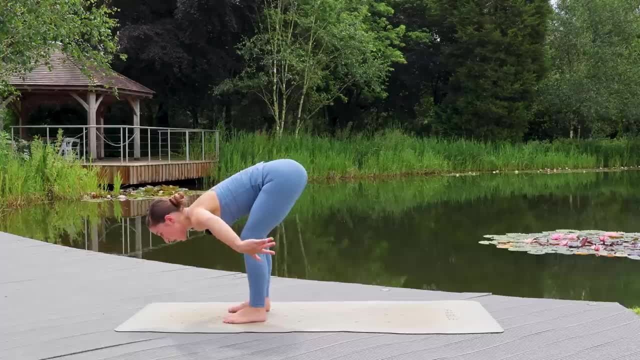 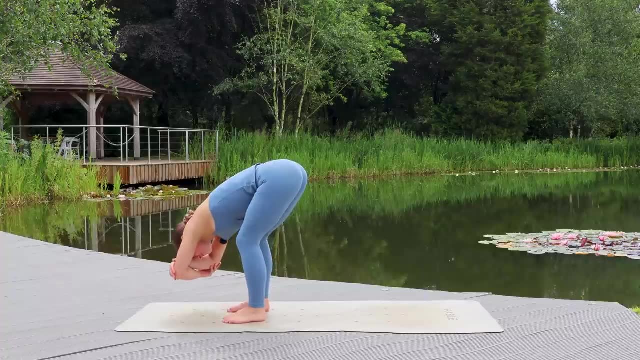 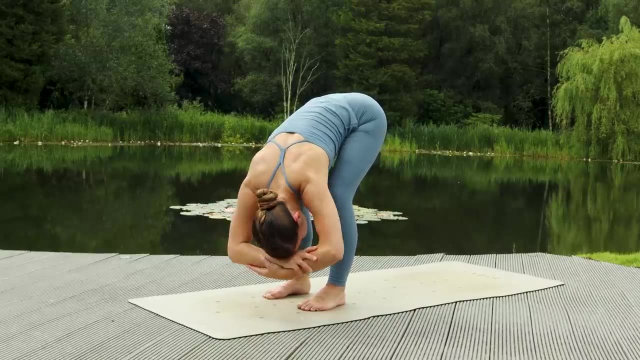 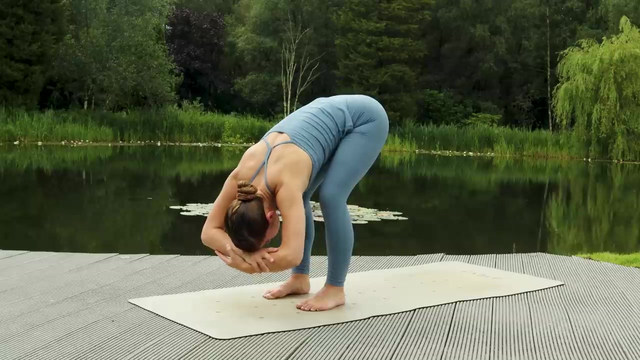 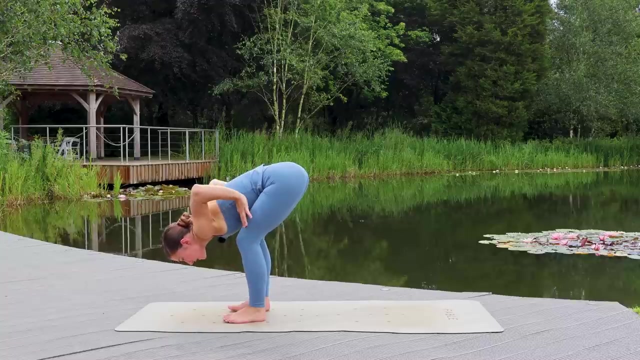 When you arrive in a forward fold, keep a bend in the knees, take opposite hand to opposite elbow and start to sway side to side in ragdoll, Letting the torso hang heavy. head and neck stays relaxed here, Good, And bring your hands to your thighs. 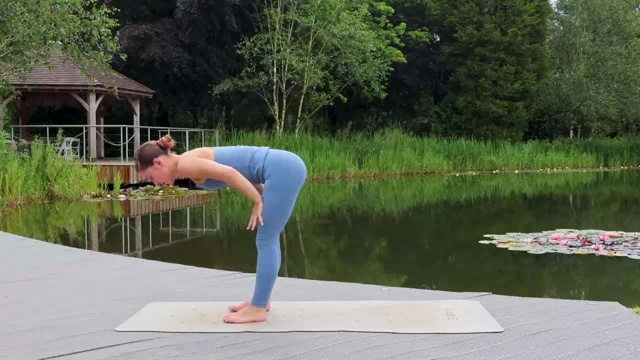 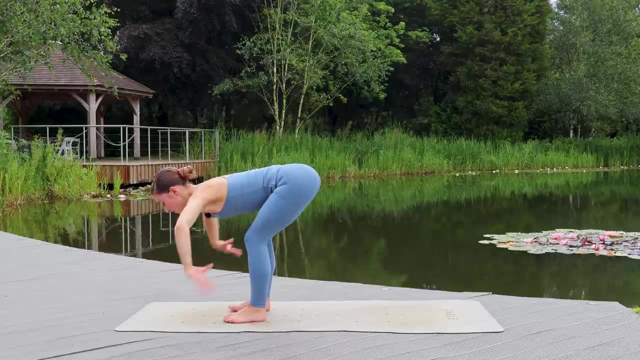 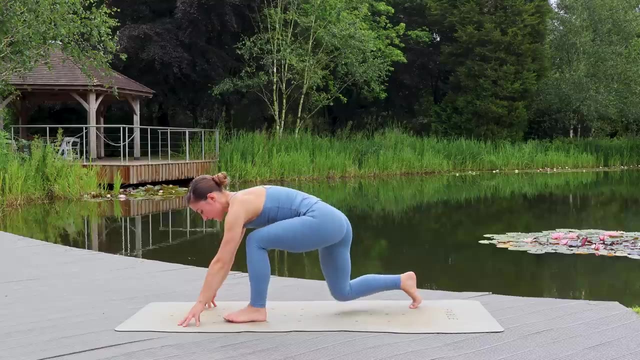 With an inhale. lift your chest halfway so that your chest is level with the ground As you exhale. fold forwards again. bend your knees so that you can bring your fingertips to the mat. Step your right foot back and lower your knee. 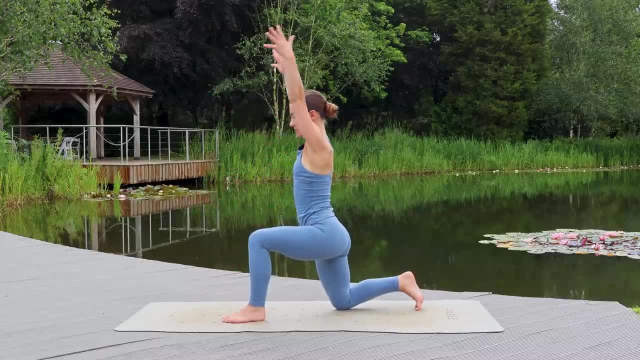 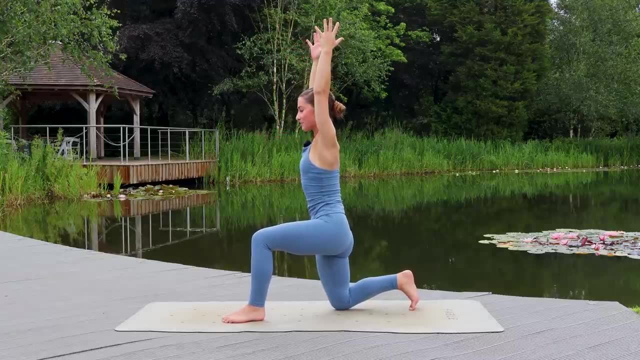 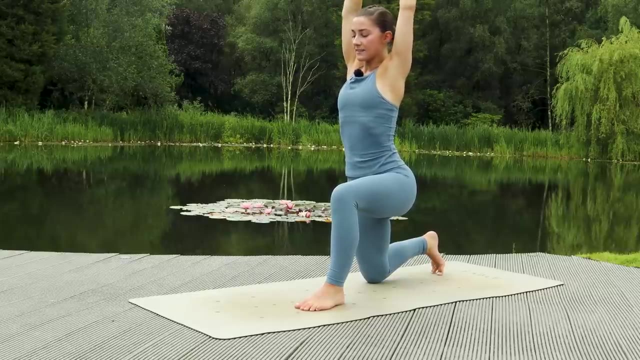 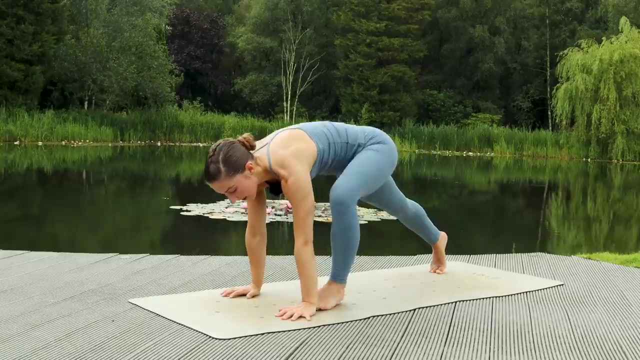 Then reach your arms up to come into lowering Low lunge. You're looking to stack the front knee over the ankle and the back knee underneath your hip. Hold for a deep breath in As you exhale. plant your hands. Start by picking up the back knee, then step your front foot back into a plank position. 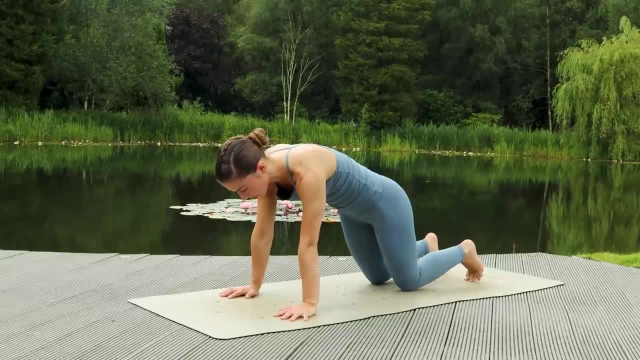 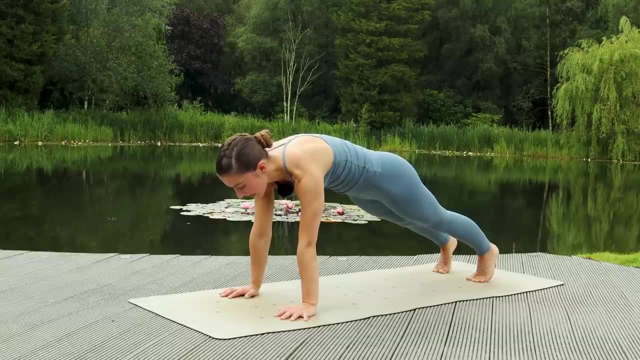 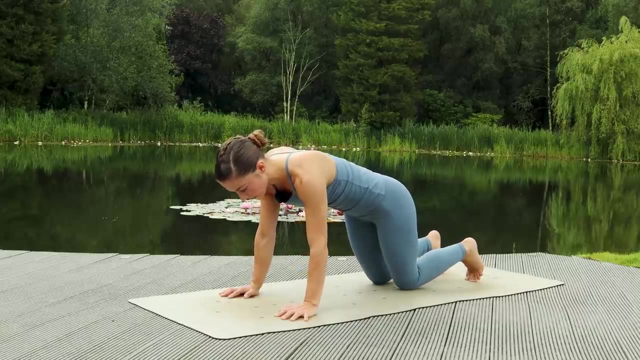 This may be quite challenging, so you could lower the knees for added support. We'll hold for a breath in, press the floor away, Exhale and lower your knees- if they aren't already. Then, bending your elbows close to the sides of your ribs, slowly lower your chest down. 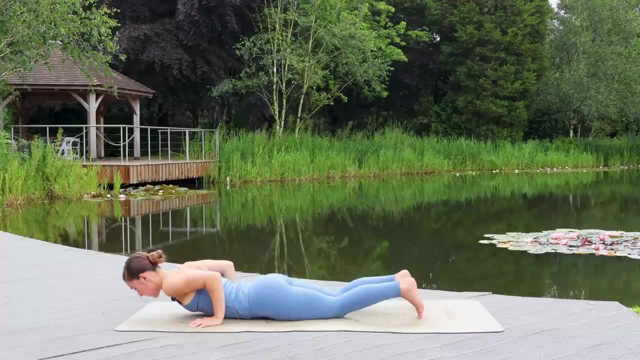 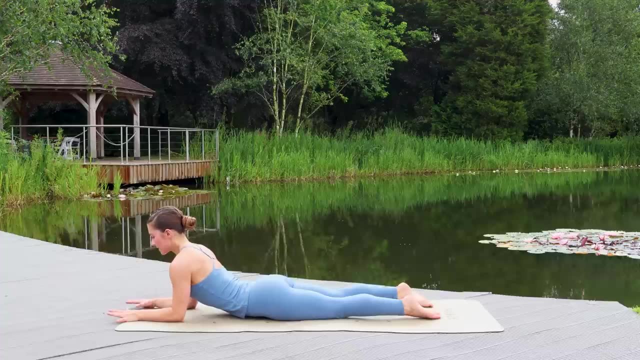 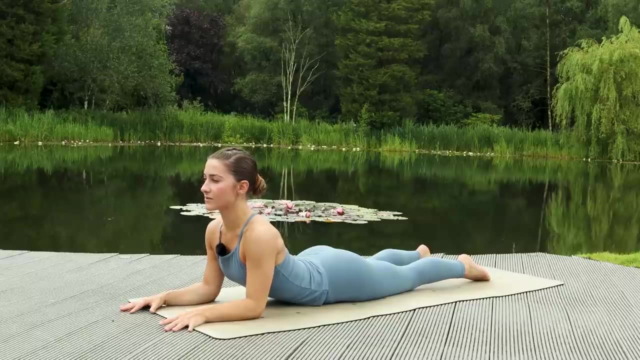 and forwards. Bring your forearms to the mat in front of you so the elbows are underneath the shoulders. Press the forearms into the mat as you lift your chest for sphinx Good, Think of rolling your shoulders back so that you open your chest towards the front of your 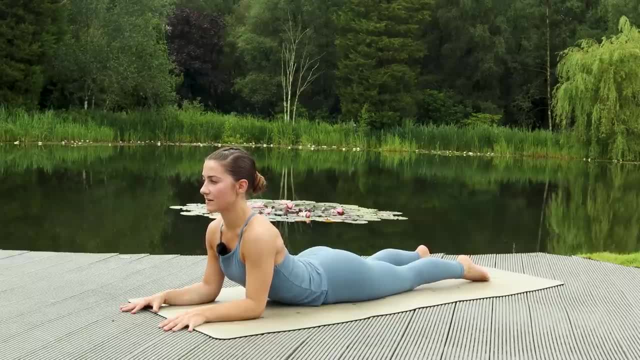 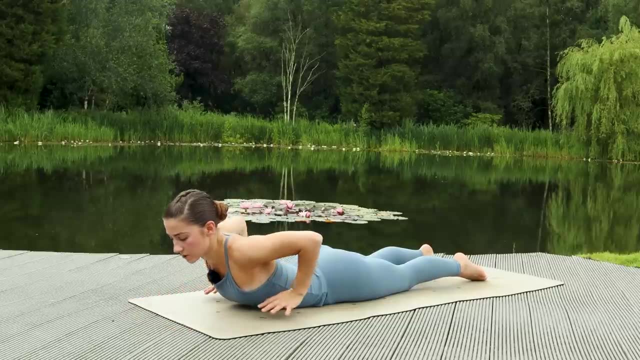 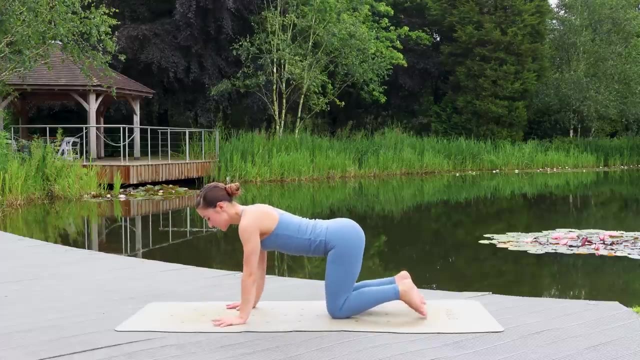 mat. Take a full breath in And, with your exhale, lower your chest, Bring your hands under your shoulders and push back up into that tabletop hands and knees position, tucking your toes Again. begin by lifting your knees, Then lift the hips. 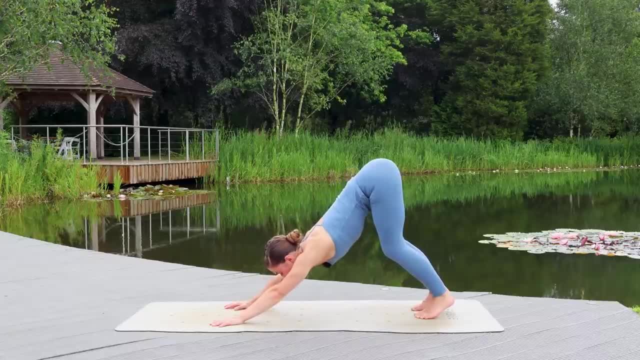 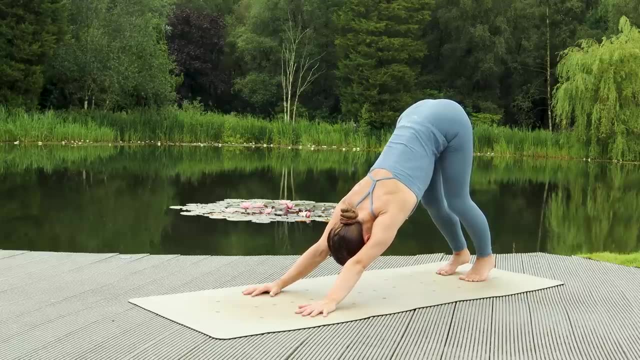 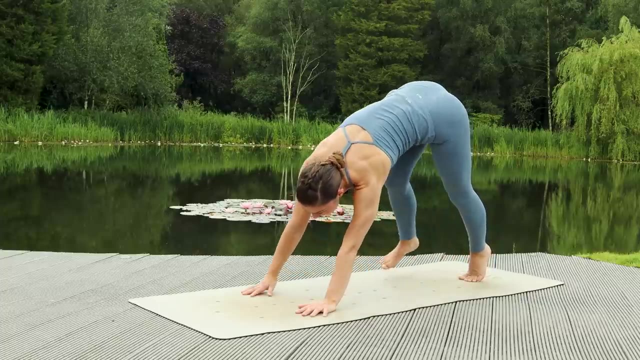 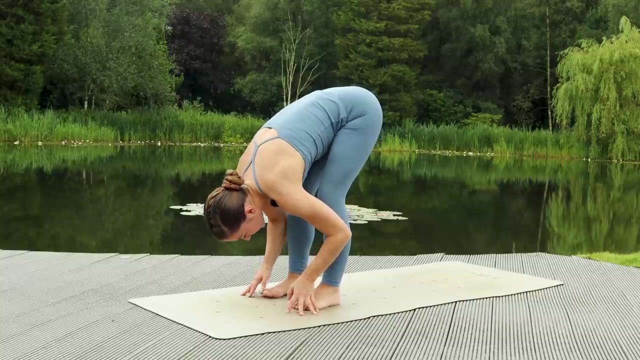 Lift yourself back, sending your weight towards your feet to come to downward dog Hold for a breath in, Exhale the breath out. Then look forwards and take baby steps to walk your feet towards your hands, Fold all the way forwards here. 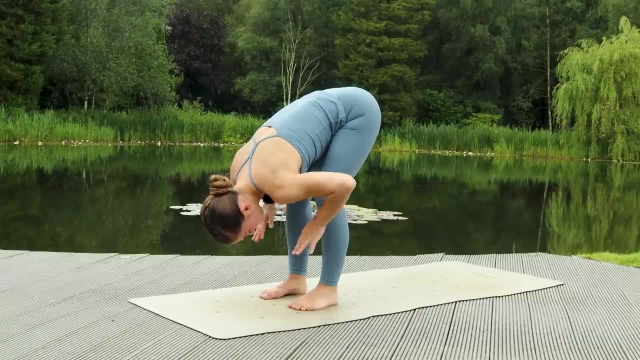 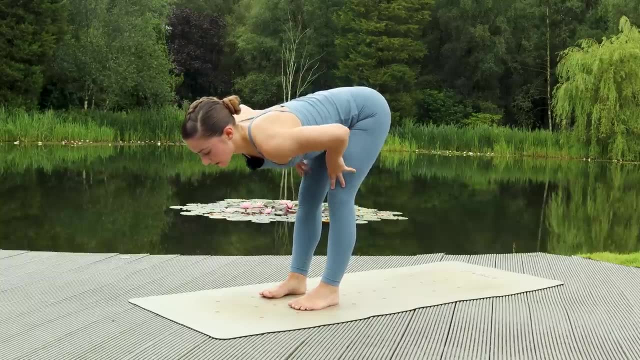 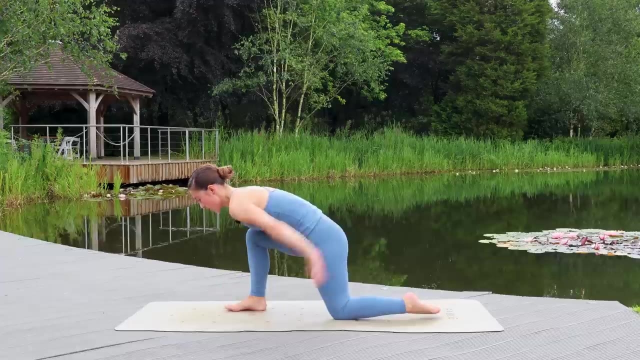 Relax your head and neck And bringing hands to thighs. inhale, lift halfway, Exhale, fold, Fingertips come to the mat and the left foot will step back. The left knee will lower down for your low lunge. 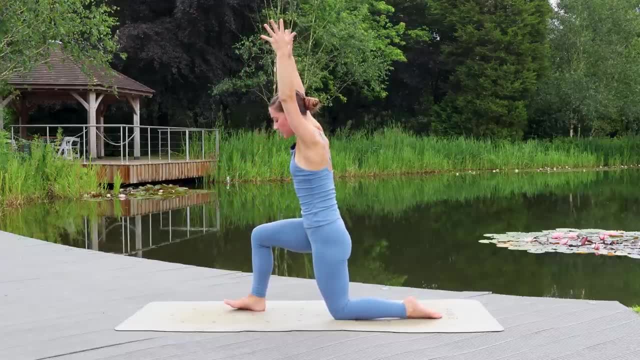 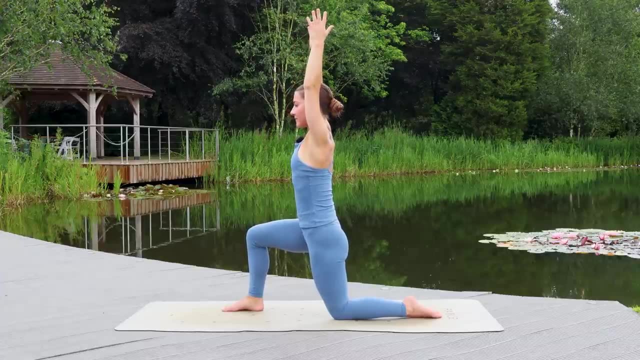 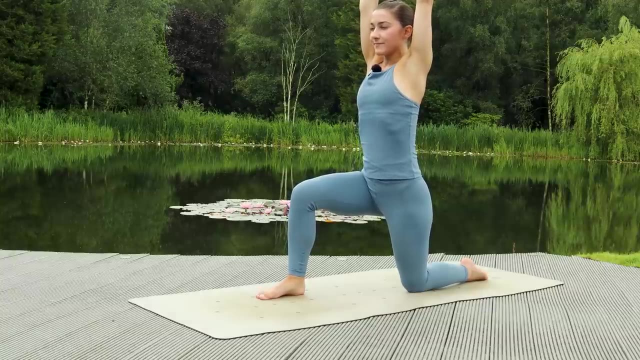 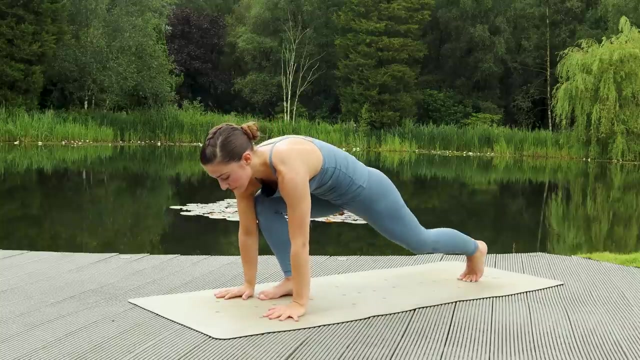 Reach your arms up and we'll take a quick alignment check. So front knee is over ankle, back knee is underneath your hips And pausing to find the breath, Deep inhale, Exhale. hands can come down. Start by lifting your back knee so that you create space to step the front foot back into. 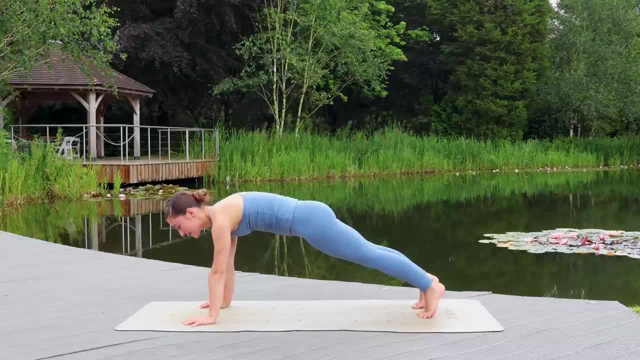 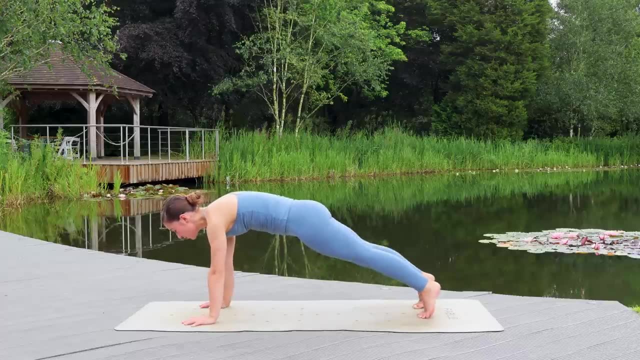 plank And you could challenge yourself here, maybe seeing if you can keep the knees lifted. If not, it's perfectly okay. if the knees need to lower down, Hold for a breath in With your exhale. lower your knees if they aren't already. 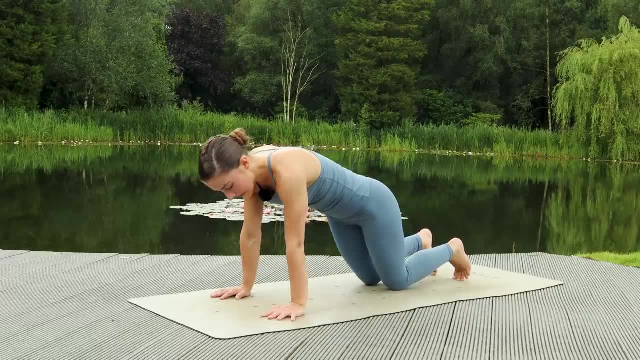 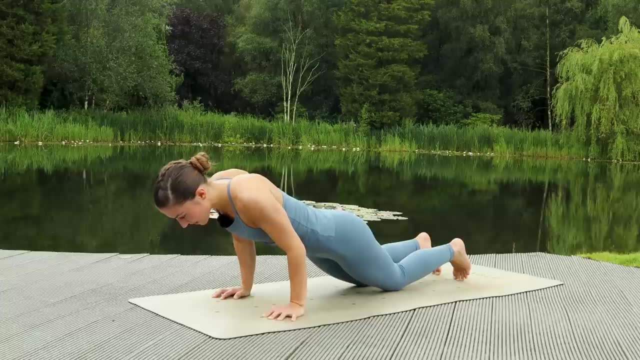 And start lifting, Then start to rock your weight forwards so you're sending your shoulders past your wrists, Bend your elbows close to the sides of your body as you lower yourself down, And you're lowering down and you're moving the body forwards at the same time. 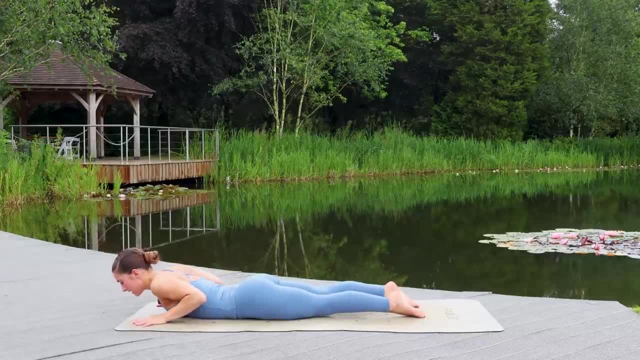 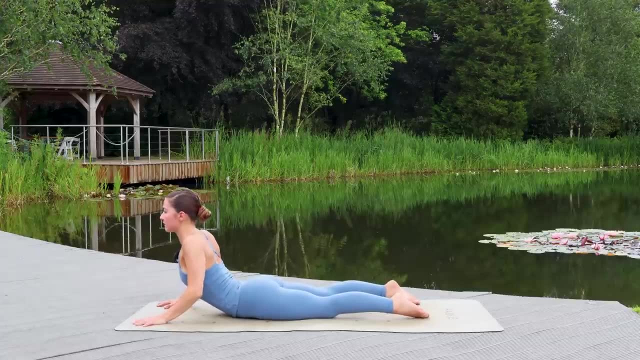 This time keep the hands under the shoulders And, with an inhale, lift your chest, Roll your shoulders back, coming into baby cobra. So it doesn't have to be a huge lift, Just lifting the chest slightly, Exhale. 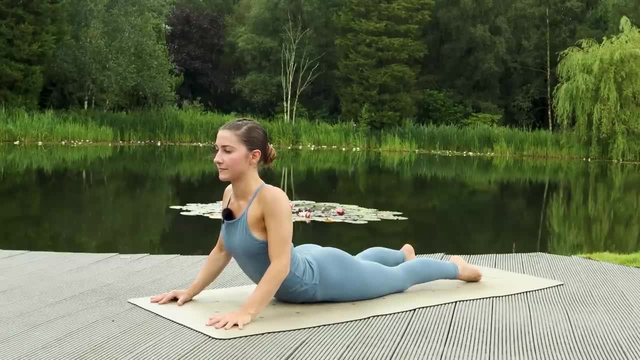 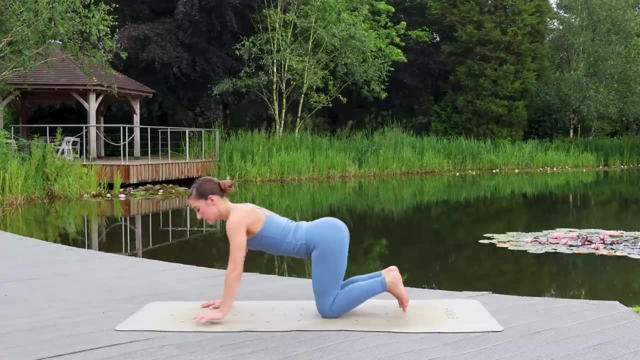 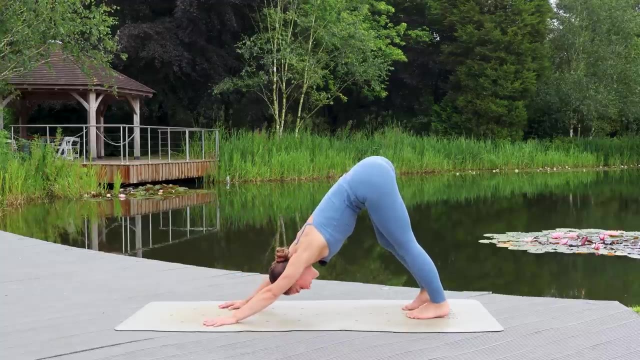 Pause for a breath With your exhale, lower back down, Come back into tabletop Again, tucking the toes, Lifting the knees, Moving back into downward dog. This time you could play around with pedaling out the legs. You're just straining one leg, keeping the other leg bent. 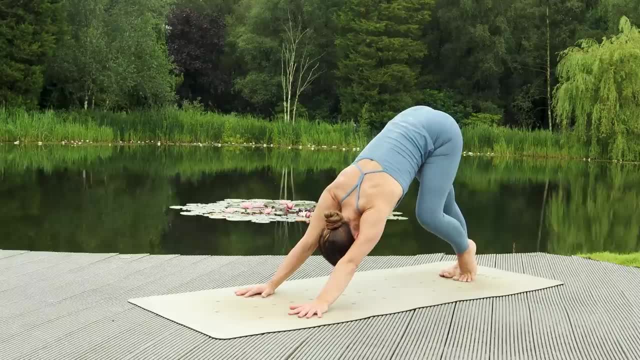 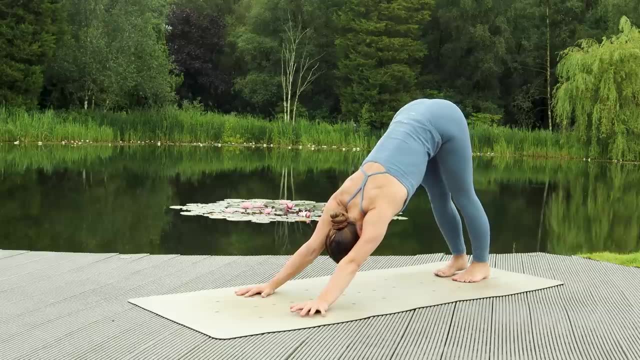 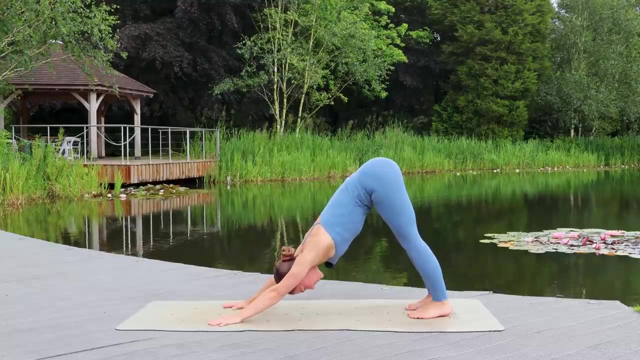 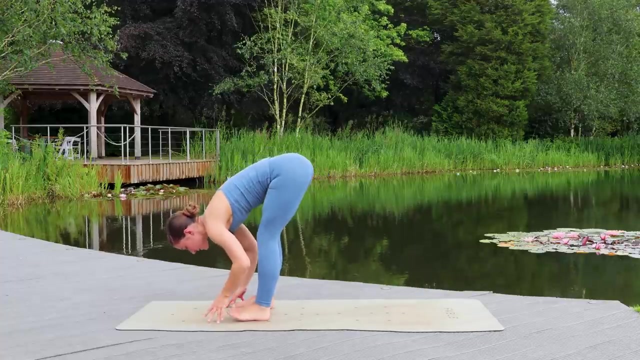 And then switching Like you're walking your legs out. Good, Good, Good. Then, looking to the top of the mat, Take baby steps, Walking the feet forwards, to come into your forward fold. Exhale all the breath out here. 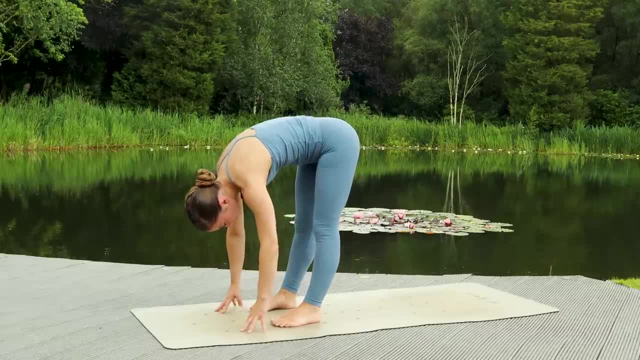 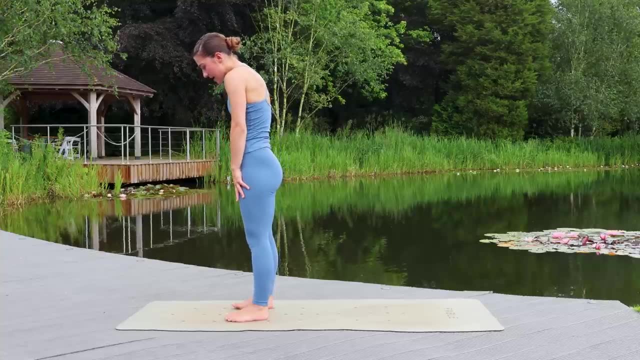 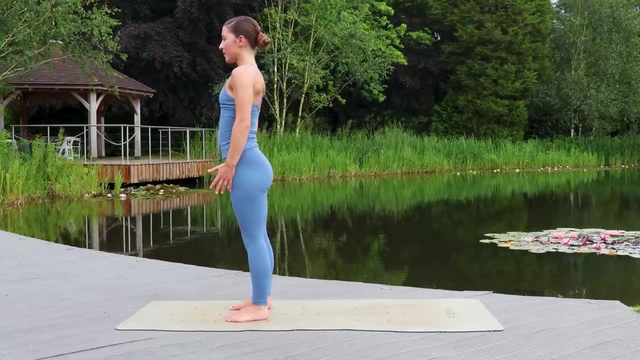 And this time we'll round the spine And slowly role all the way up into a standard plank, A perfect plank. My ballet is clothes standing position. So you're just slowly stacking the spine to stand tall, Keeping the feet hips width On your inhale. reach your arms up and start to bend your knees and sit your 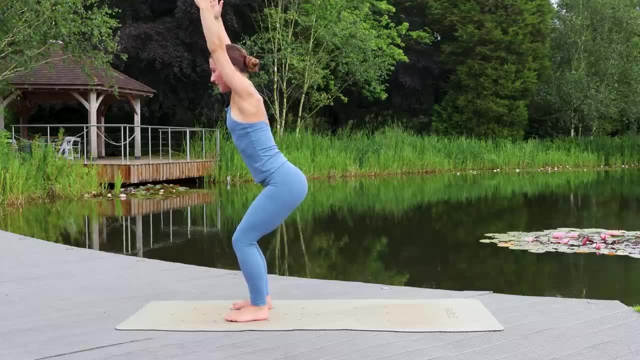 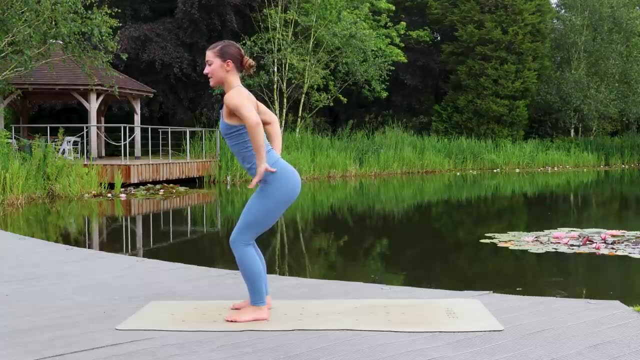 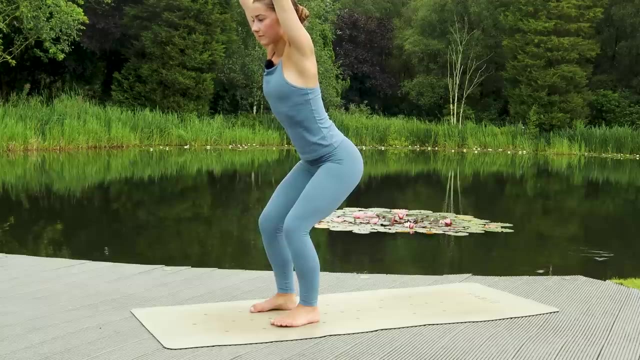 hips back like you're sitting back in a chair. There can be a temptation here to stick your bum out, So try to tuck your tailbone under slightly to keep the lower back nice and long. Keep shifting your weight back through your heels. See if you can go just a touch lower. 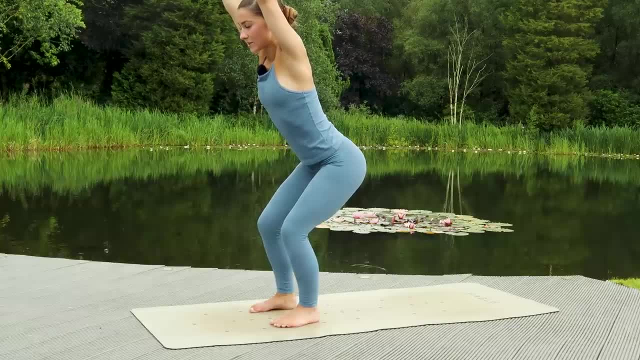 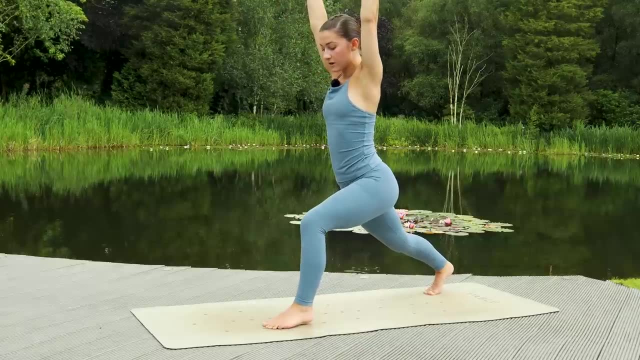 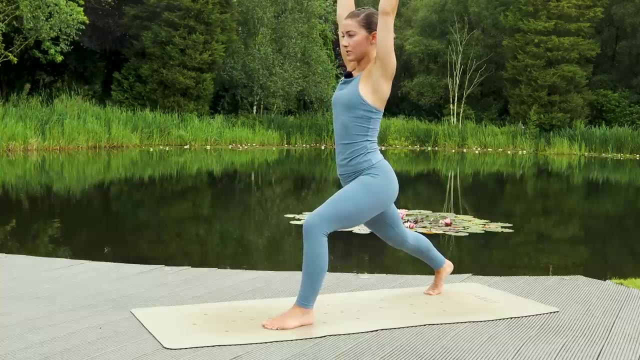 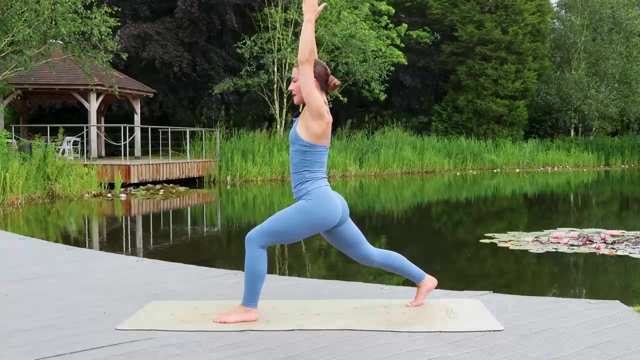 And take your weight into your left foot and slowly step your right foot back, coming into high lunge. Similar to low lunge: the front knee is over the ankle, but this time the back leg is straight and you're just up on the ball of your foot. Hold for an inhale. As you exhale, turn the. 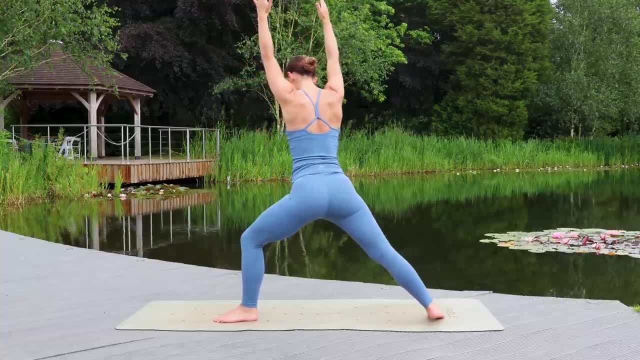 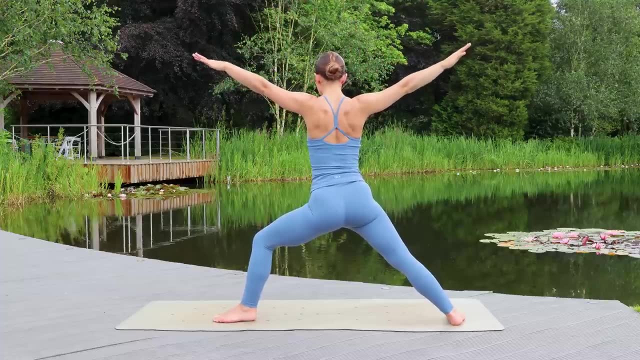 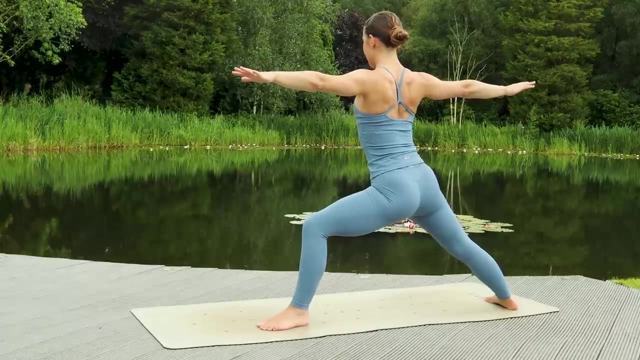 back foot open, so you're lining up the middle of your back foot with your front heel, turning your body to the side and opening the arms into a T-shape. As you open the arms wide, relax your shoulders down your back, away from your ears, Then, gazing forwards, flip. 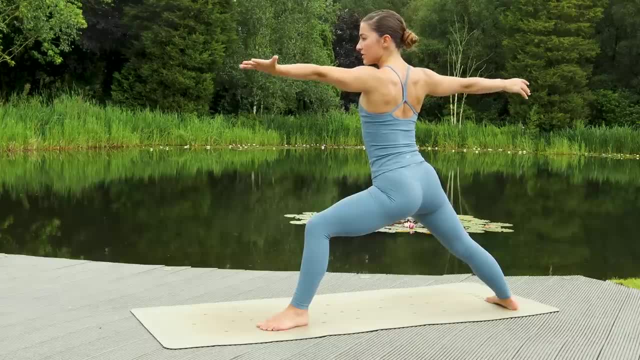 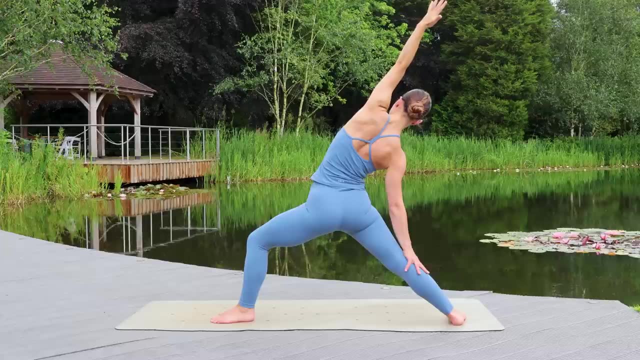 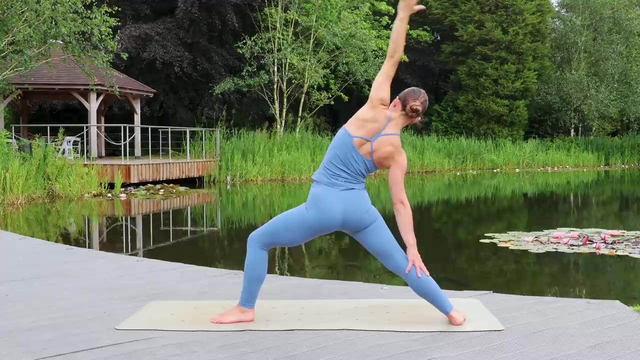 your front palm to turn up. Reach the front arm up as you lean back and your right hand can rest on the back leg. Take a full breath in here As you exhale. come back through to your warrior two. Rest the left forearm on the thigh. 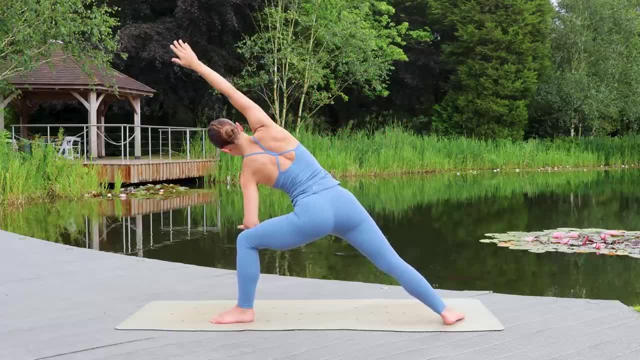 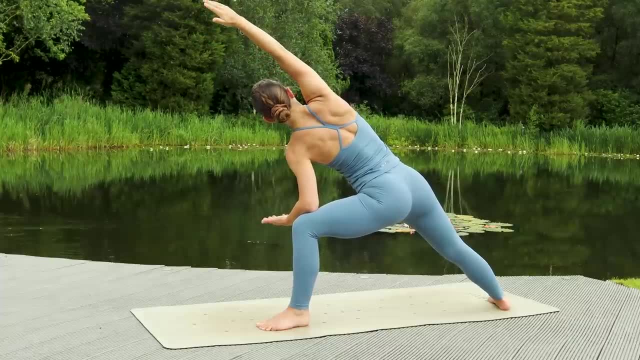 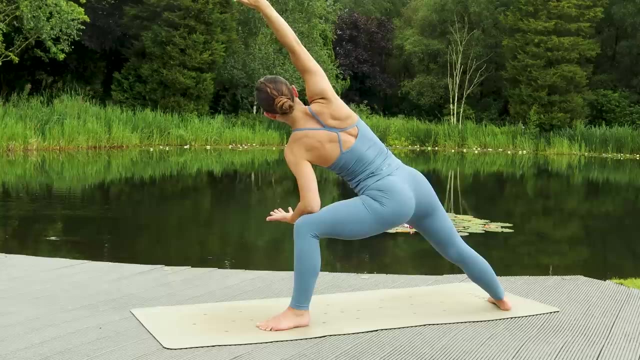 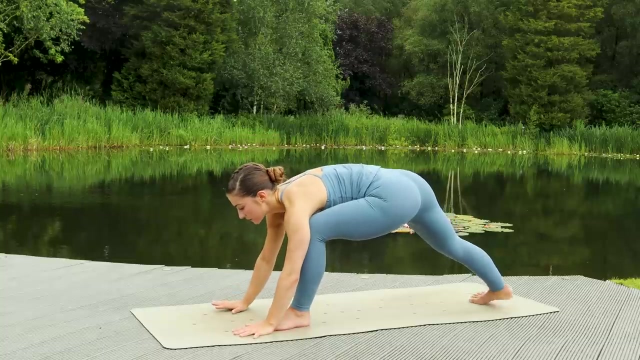 And reach the right arm overhead towards the front of your mat. As you hold this, turn your chest open slightly towards the sky. Take a full breath in, Exhale out. Then, looking down for balance, place both hands down, Turn the back foot to face forwards and step to. 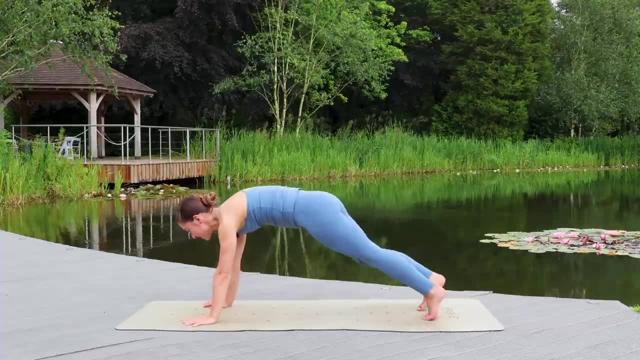 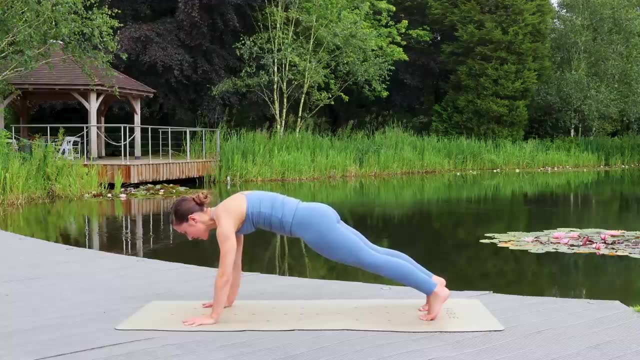 plank. Maybe challenge it a little bit. Imagine yourself this time to keep the knees up. If not, you can always lower them down. Hold for a full breath in pressing the floor away. As you exhale, the knees will come down. 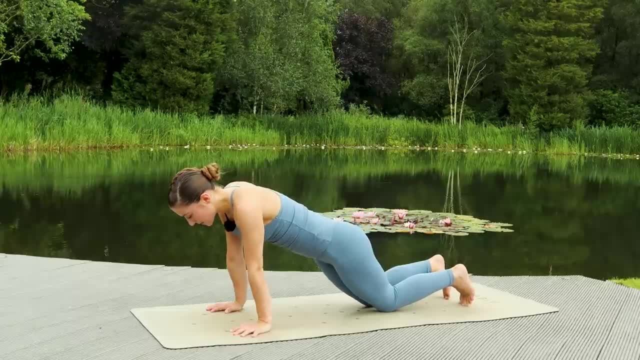 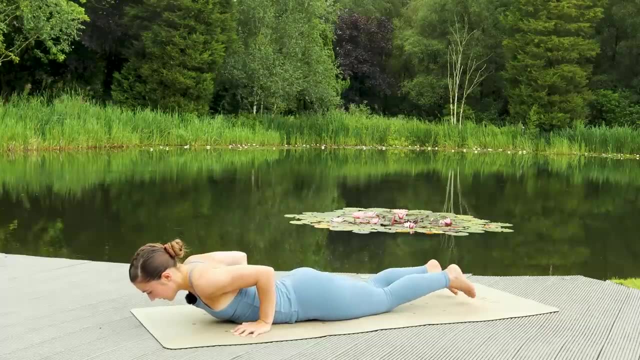 Just like before, start to shift forwards, Bend the arms, keeping them close to the sides of the body so they're not winging out to the sides, and lower down to your chest. Keep the hands under the shoulders. Inhale to lift your chest. Maybe this time you go a little. 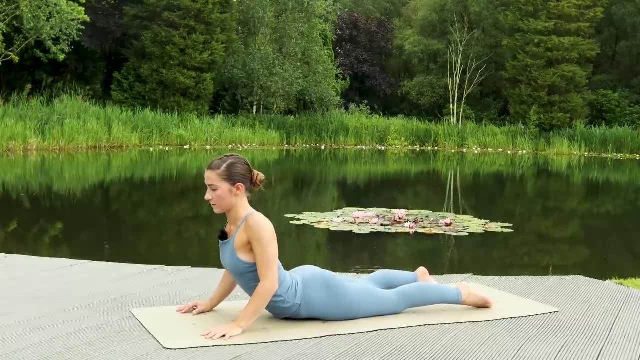 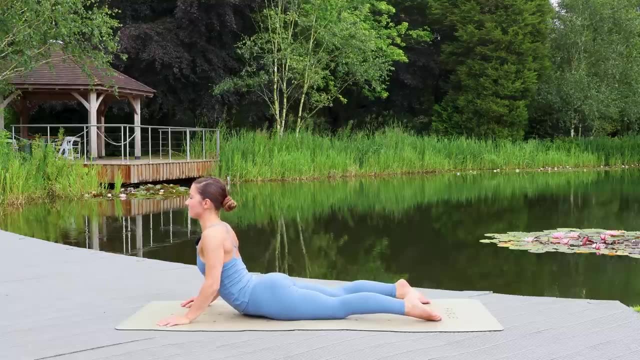 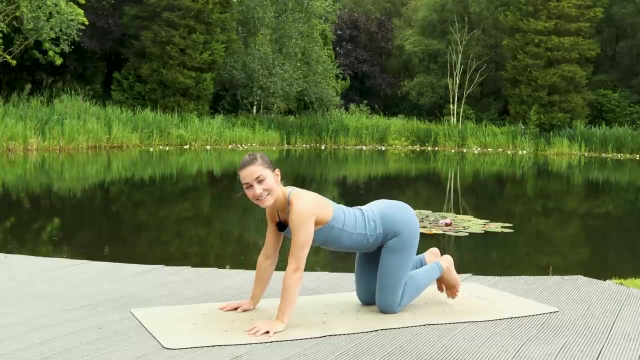 higher into your cobra. but there's no pressure if not, Roll your shoulders back, big breath in, exhale, slowly lower down, push back into your tabletop and come all the way back into downward facing dog Again. you can stay in stillness or 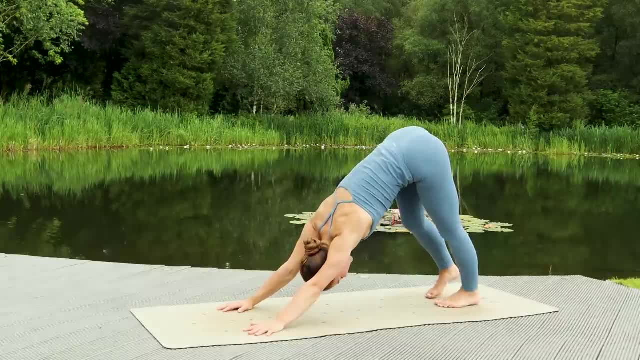 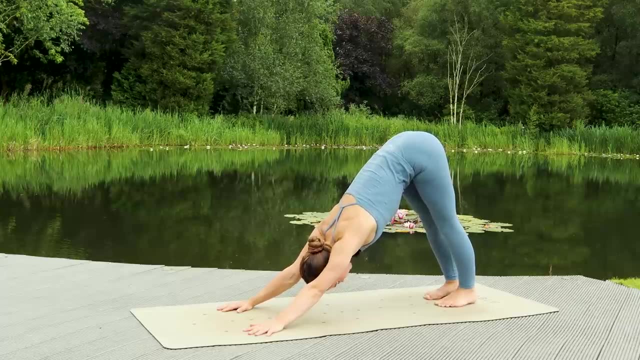 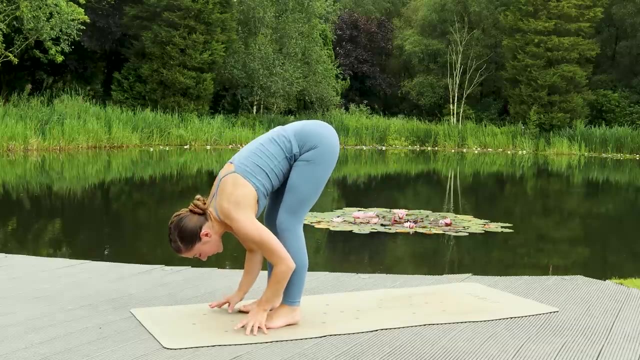 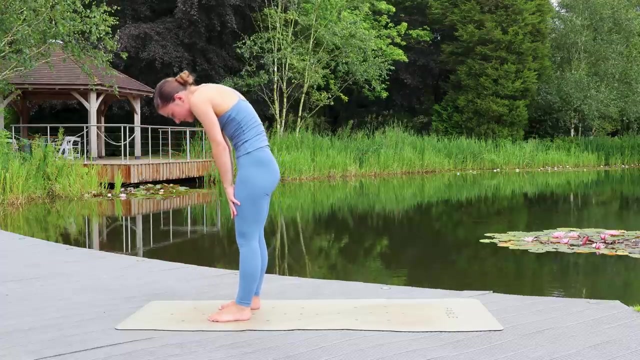 you could play around with pedaling out the legs, just finding what feels good in your body. Then, looking forwards, take baby steps to the top of the mat and exhale in your forward fold, Rounding the spine, roll all the way up to stand and 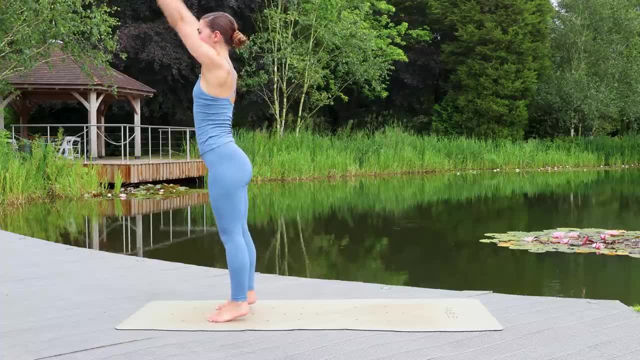 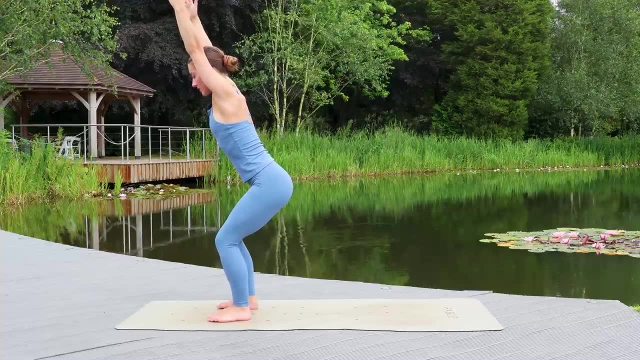 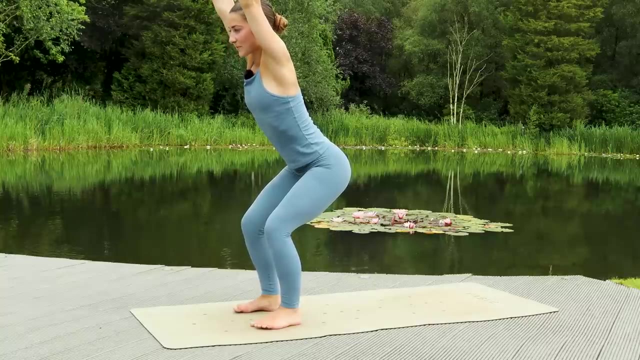 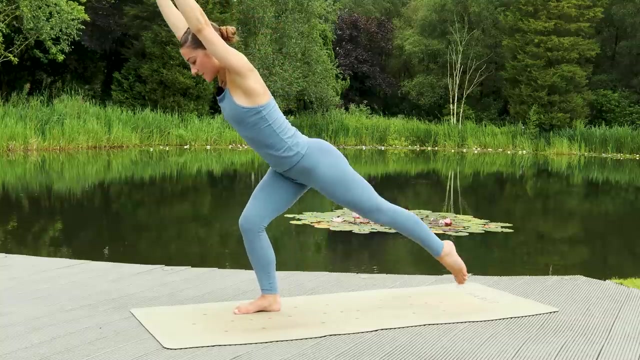 reaching your arms up as you bend your knees. lower your hips into your imaginary chair, Keeping the lower back nice and long. shift the weight back through your heels. see if you can go just a little bit lower, Great work. Shift the weight into the right foot as you slowly step the left foot back into. 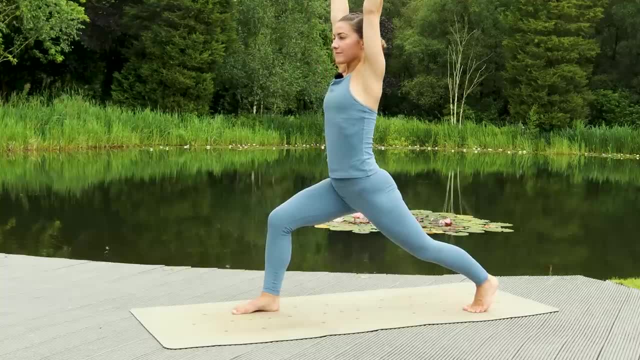 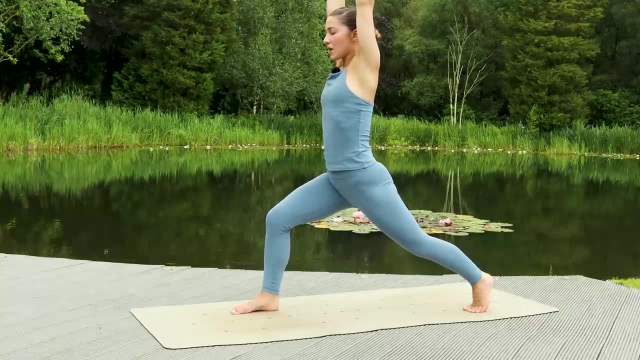 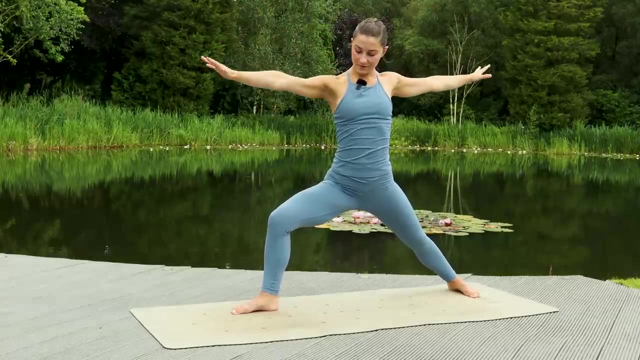 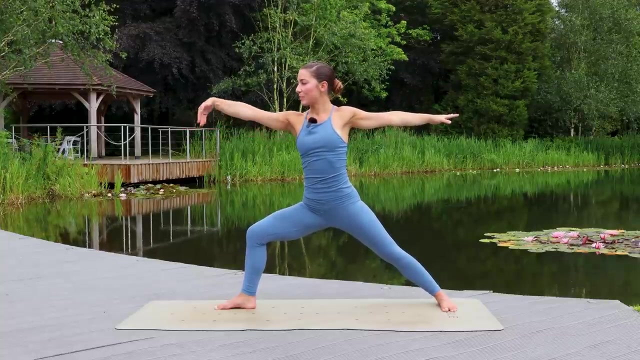 your high lunge. Take a full breath in as you exhale. open out your back foot, turn your body to the side. open your arms to a T-shape- You can relax your shoulders away from your ears and flipping the front palm to face up. Inhale, reach the. 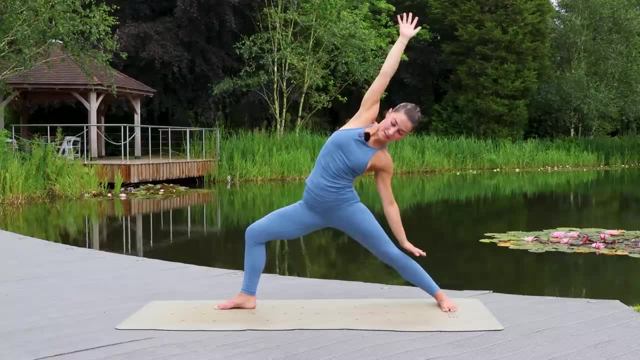 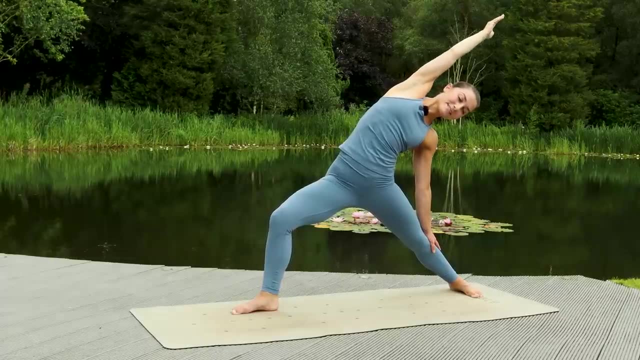 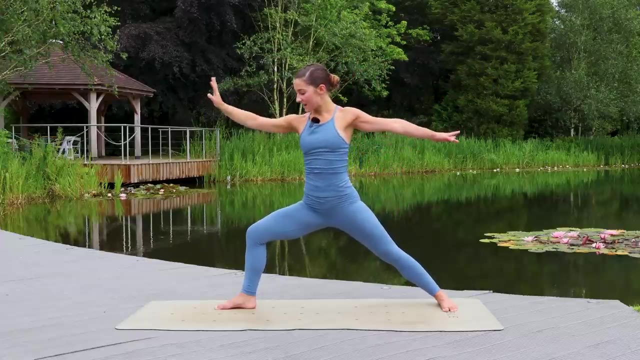 right arm up. as you lean back, Left hand can rest on the leg. Hold this position, reaching the right arm all the way up to the sky With your exhale. return through warrior two. Then rest the right forearm on the thigh. Left arm will reach overhead. 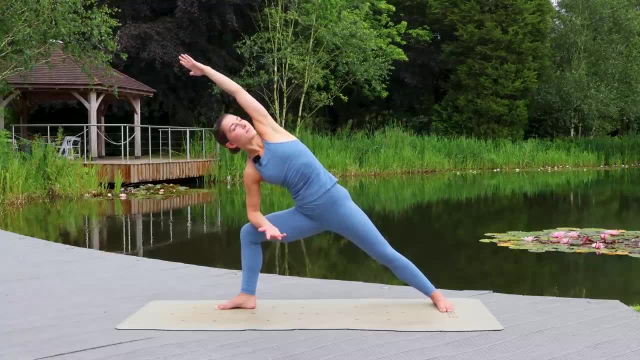 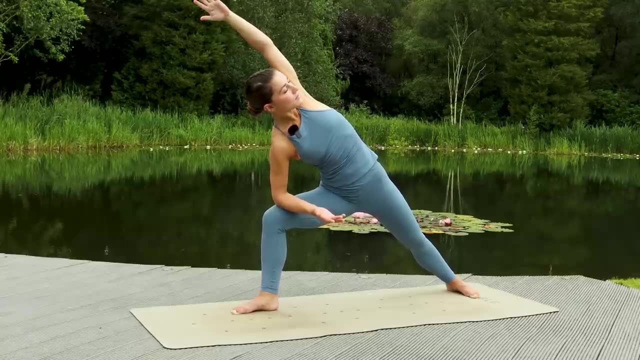 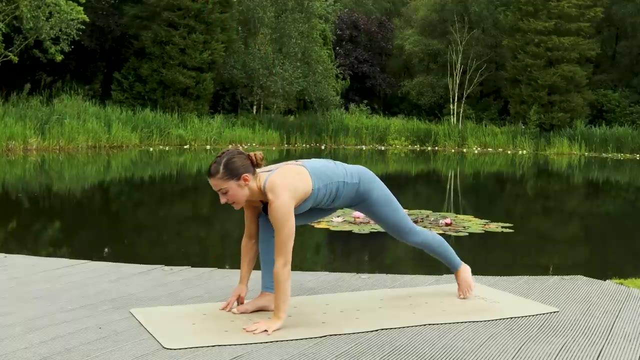 And you're looking to turn your chest open to the sky. Take a full breath in, Exhale the breath out, Then look down for balance, Bring your hands to the mat and step back to plank, Challenging yourself as you press the floor away from the mat. 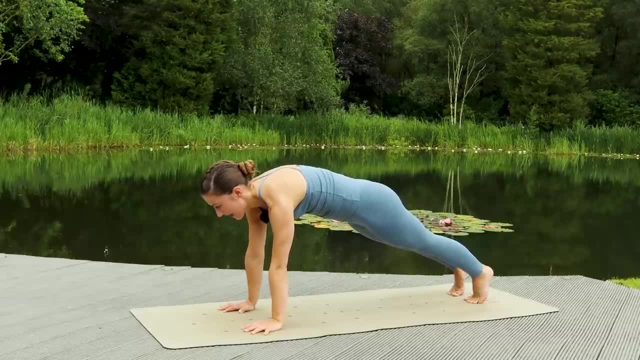 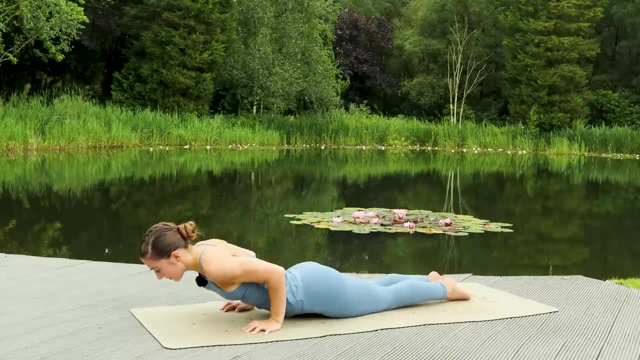 Challenging yourself as you press the floor away from the mat. Challenging yourself as you press the floor away from the mat. Challenging yourself as you press the floor away. Big breath in Exhale. knees down, Rock forwards, bend your arms lower down to your belly. 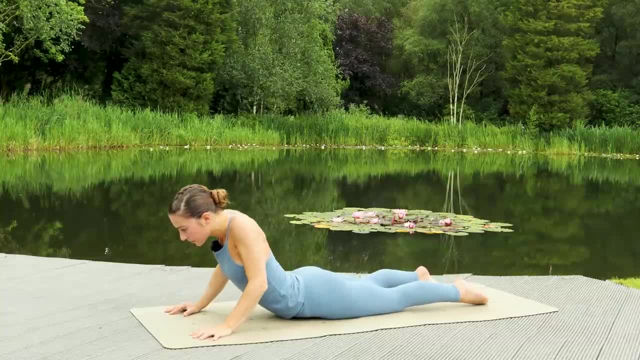 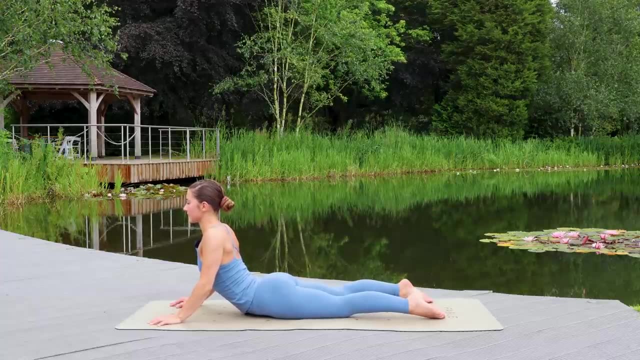 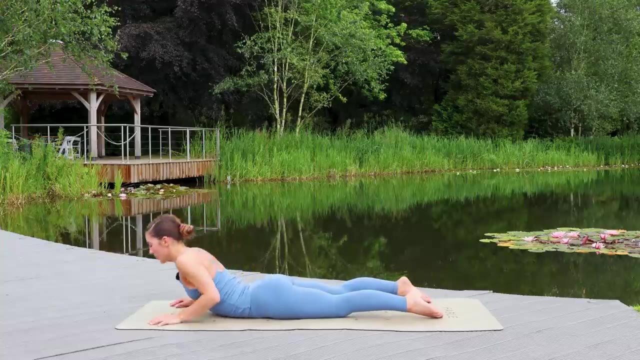 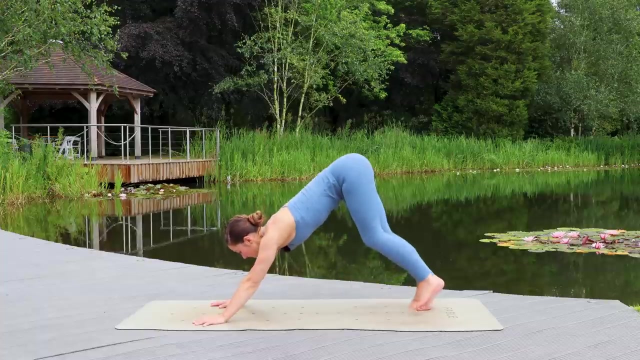 Bring hands under shoulders. Inhale and lift your chest for cobra, Rolling the shoulders back as we pause a few moments here And then lower the chest. Press both of your hands back into your tabletop, Tuck your toes. lift your hips into downward dog. Take a full breath. 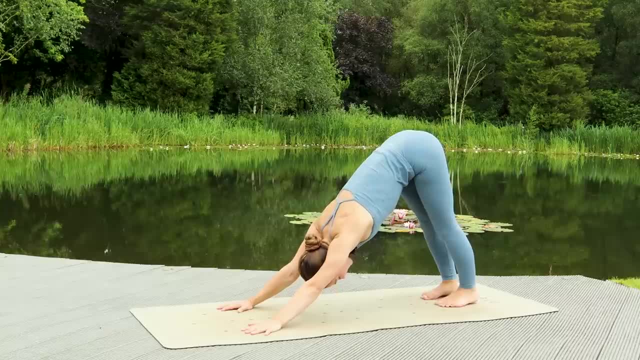 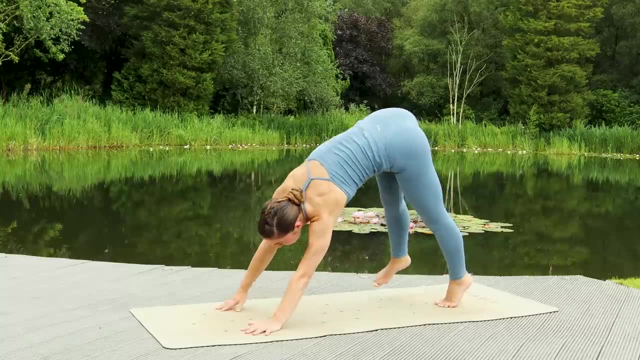 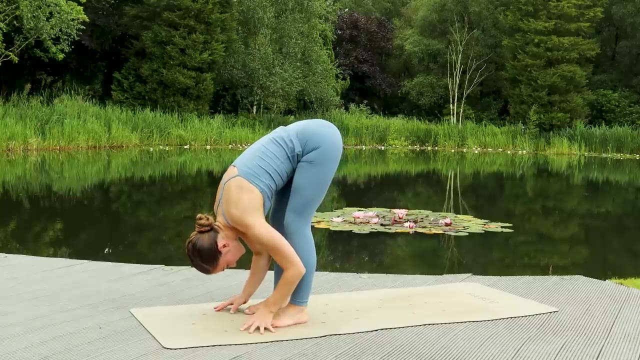 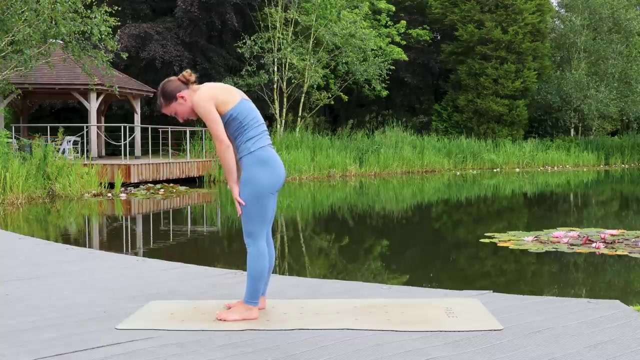 in through your nose, Exhale through your nose or mouth. Looking to the top of your mat, you can take baby steps to walk the feet forwards, Exhale all the breath out in your forward fold, Then slowly round your spine, roll all the way up to stand, Relaxing the 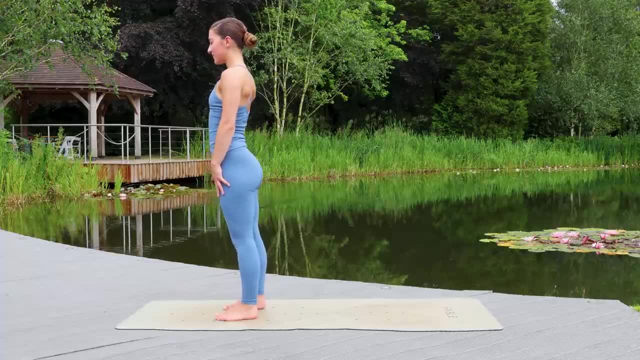 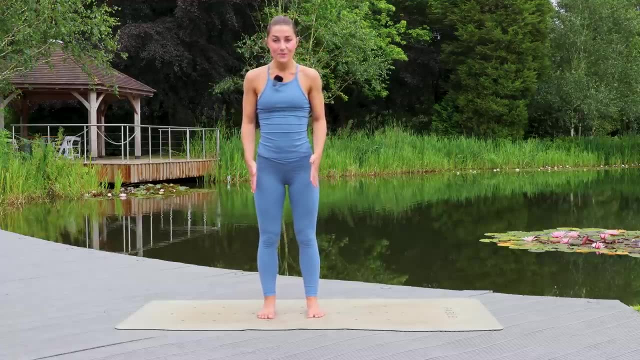 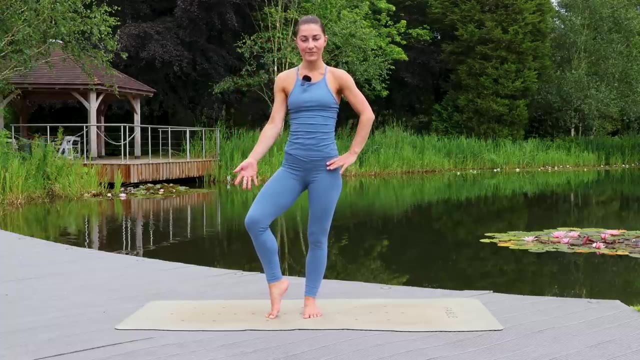 shoulders away from the ears. as you stand tall, Then I'll turn side on so that you get a better view. Keep your feet hips width for stability. Then start by lifting the right heel and opening the knee out to the side. As you do this, you can rest the right heel. 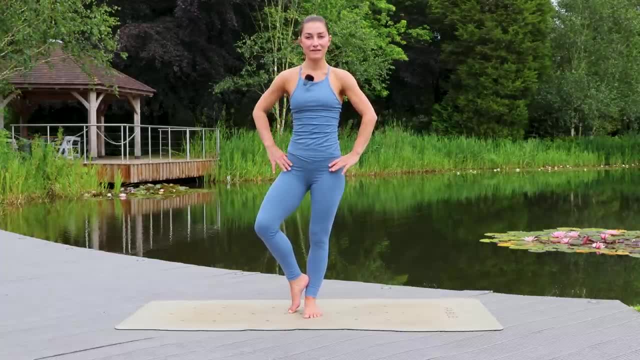 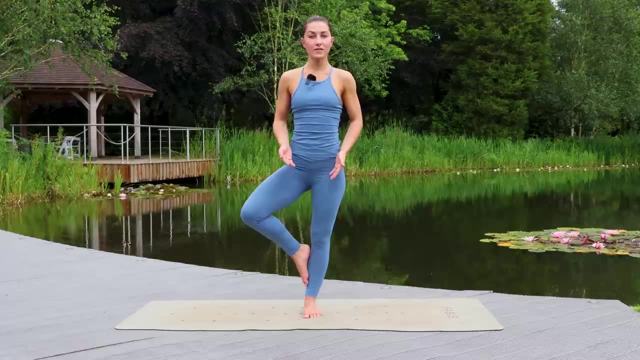 right up against the lower inner left leg for your tree pose. If you are finding that you're feeling quite balanced, then you could lift the foot up the lower leg so it's resting just below the knee. If you are feeling quite balanced still, then you could lift the foot. 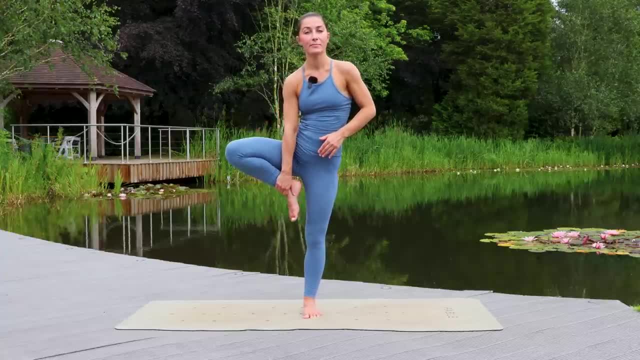 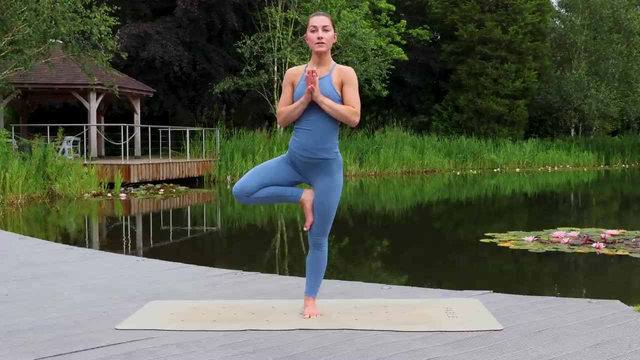 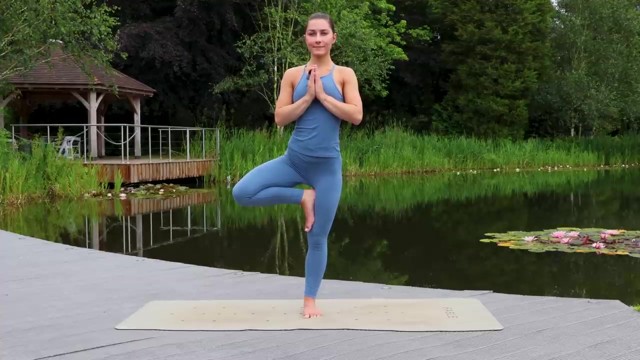 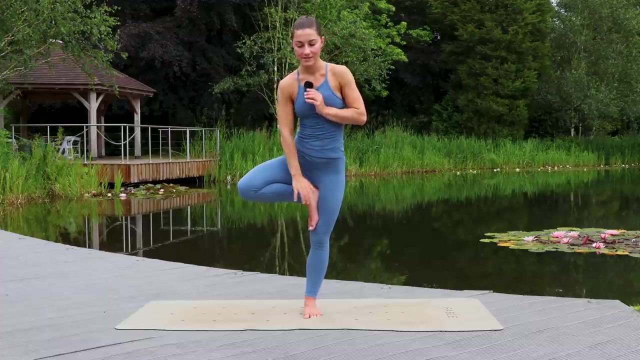 and bring it above the knee and you can use your hand to place the foot in place. Then your hands can come to prayer. Focus your gaze on one spot and slowly lift the foot to the other side. Let your breath flow. Then we'll release. You may find that you 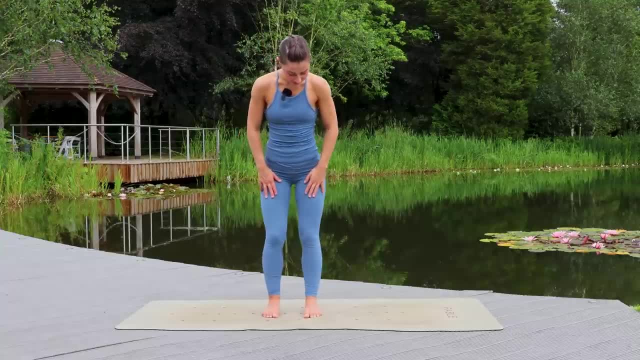 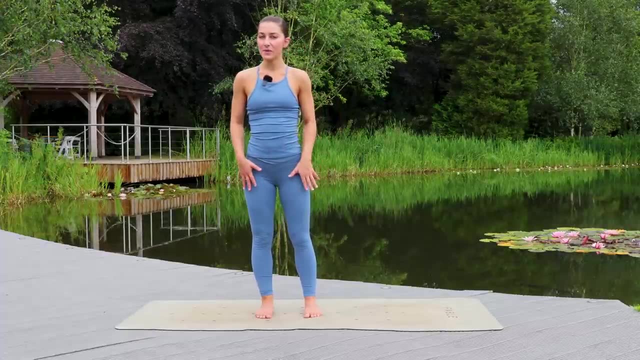 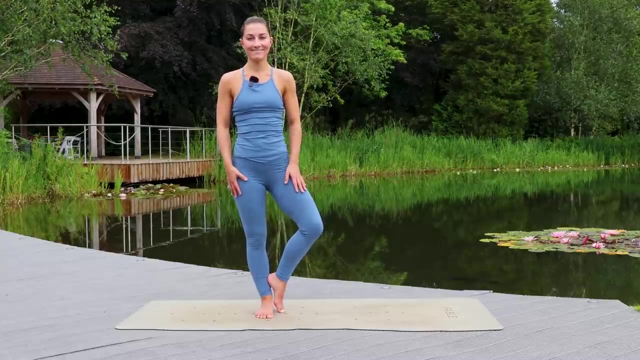 need to pedal out the legs. Sometimes it can help after balancing on one foot. Then we'll shift to the other side. So you can start by picking up the left heel, turning the knee out to the side and resting the heel against the lower right leg. If that's feeling good, you may like to experiment edging. 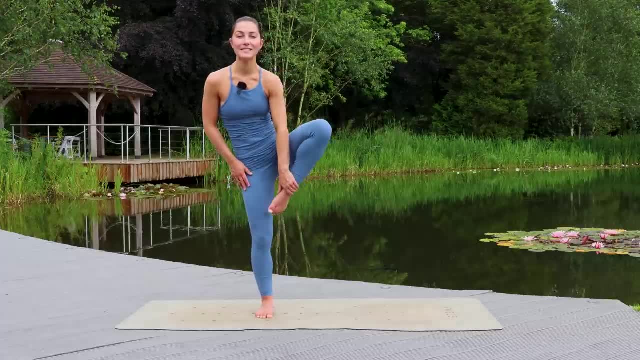 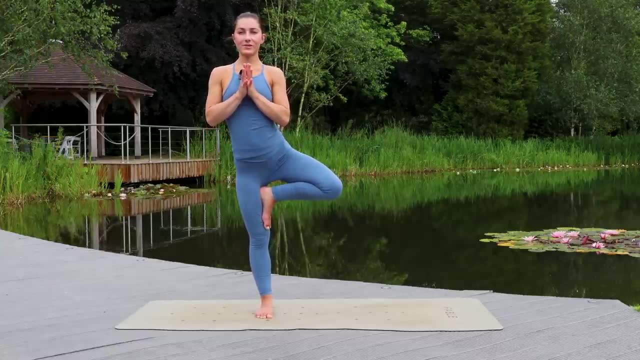 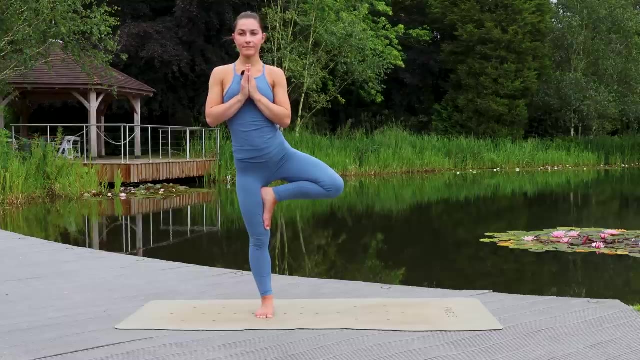 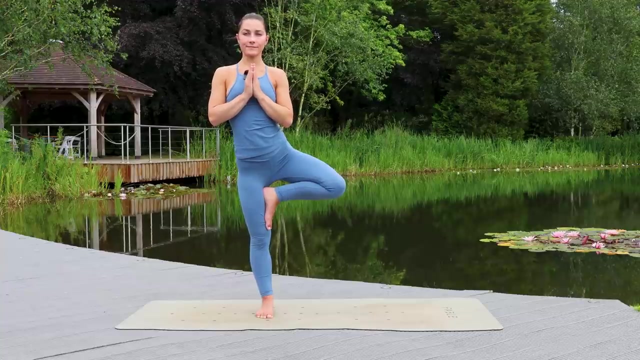 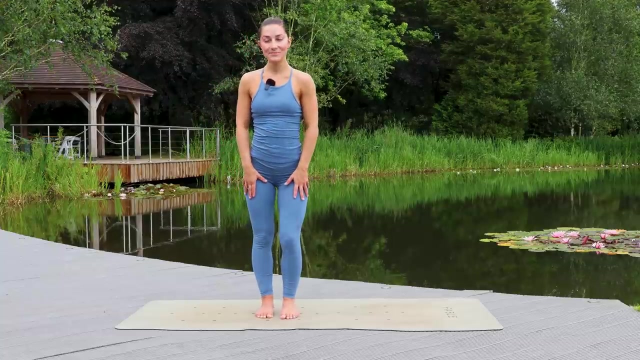 the foot up the lower leg or maybe even placing the foot above the knee. Hands. come to prayer again, slowing down the breath as we pause in our tree pose Slowly, release the foot, Walk out the legs if you need to, Then step your feet as wide. 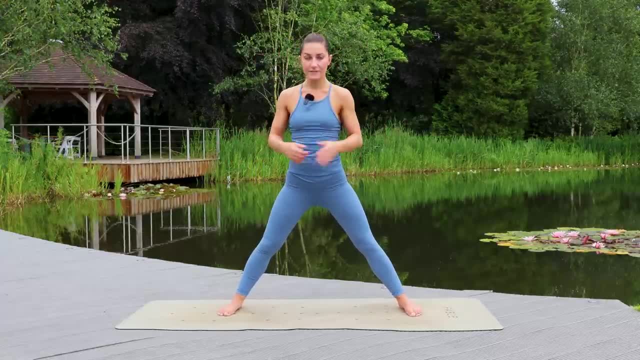 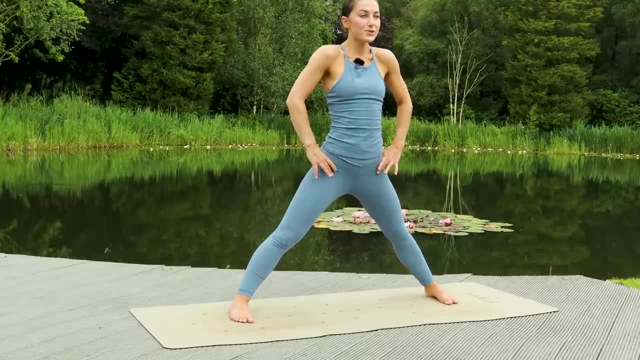 as your mat. So if you are still facing the front of the mat, you may prefer to face to the side so that you have more space. Keeping the hands at the hip creases, inhale, roll your shoulders back And as you exhale, 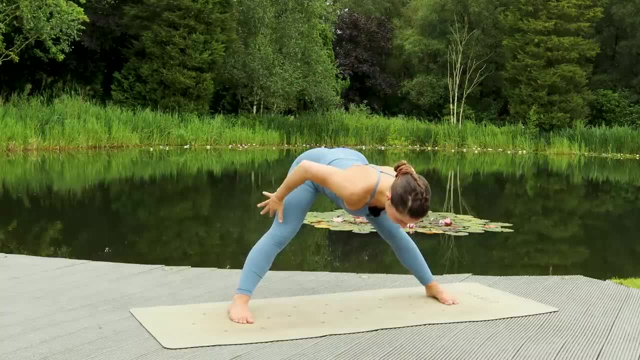 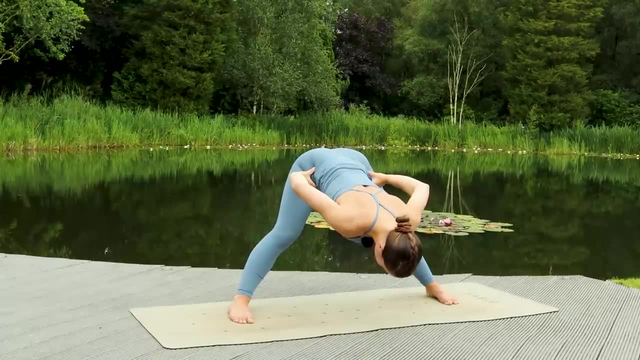 fold forwards. As you fold, you may find that you need to keep a slight bend in the knees to make it more accessible. That's perfectly okay, And you have the option to keep the hands on the hips or you could bring the hands down to the mat or a set of blocks. 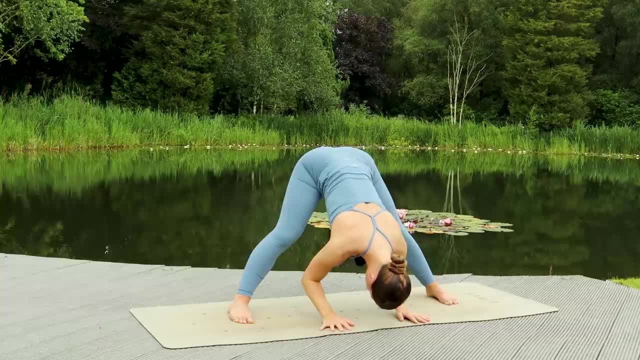 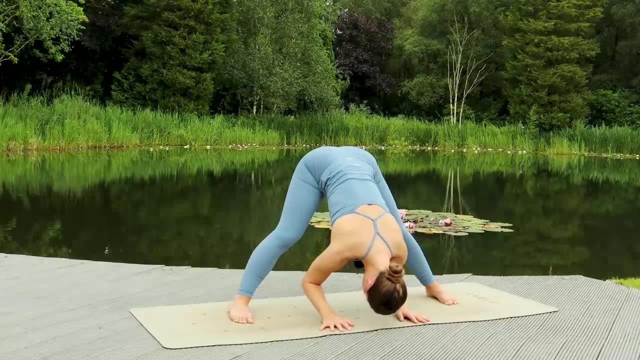 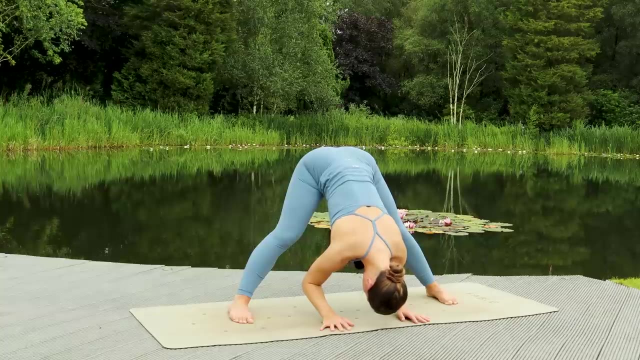 if you've got them, Just letting the upper body hang heavy. so gravity is doing the work. You're not just thinking about what you're actually doing. Take them off the mat And now lift your chest up. Inhale and lift the chest up as you exhale. 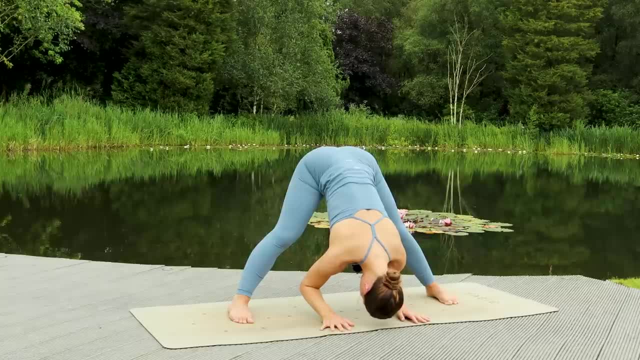 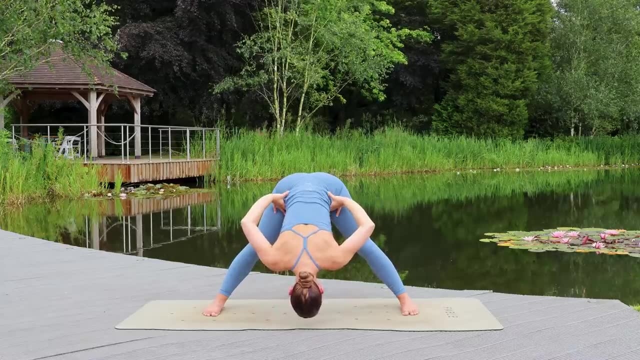 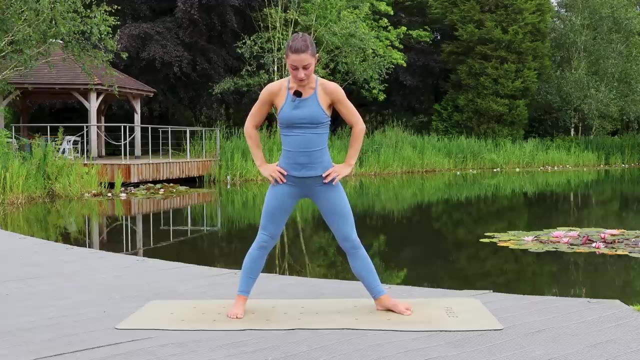 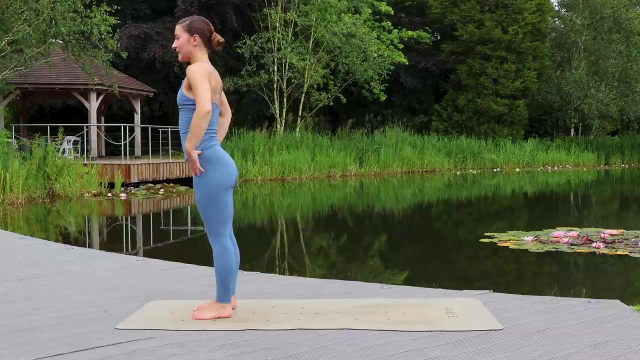 And then inhale. Bring your hands to your hips- if you took them to the mat or block, Inhale and lift the chest up. Then you can walk your feet into a立 갖 together. Come and stand at the top of your mat With an inhale. reach the arms up As. 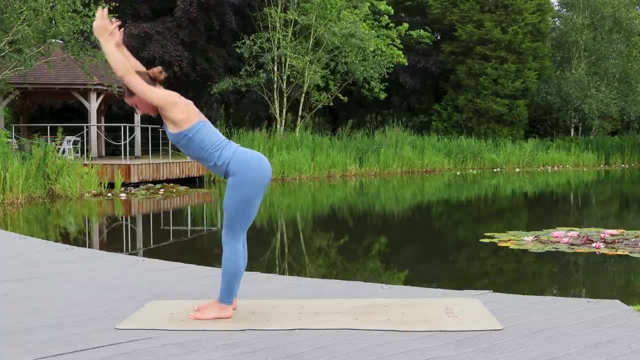 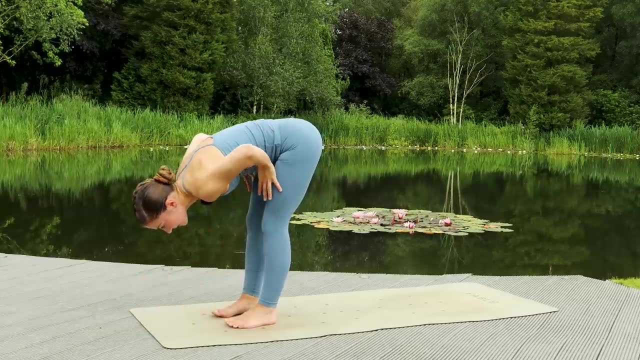 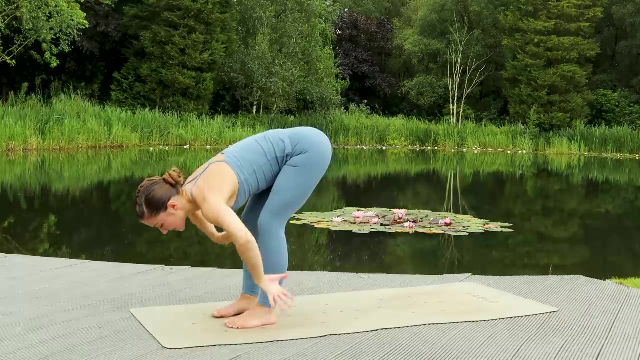 you exhale, hinge from your hips and fold forwards So you could keep a bend in the knees as you fold And hands can come to thighs. Inhale, lifting the chest halfway. Exhale: we'll fold all the way forwards, planting the hands, stepping both feet back to plank. 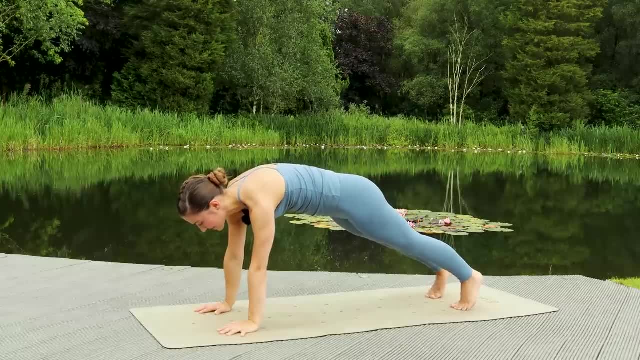 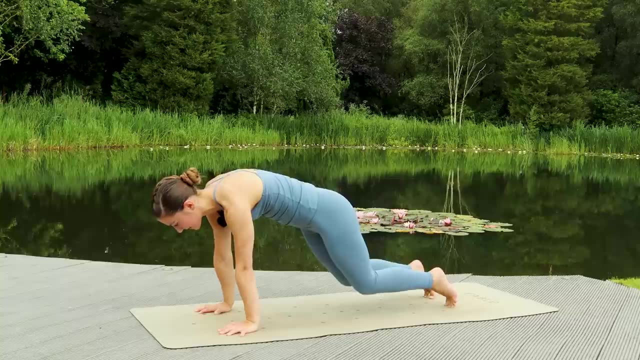 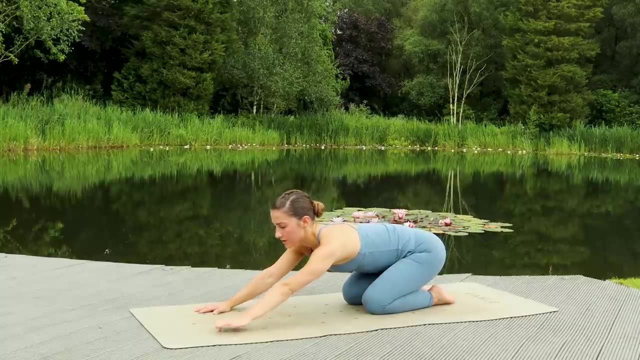 When you come to plank, hold for a breath in See if you can challenge yourself one last time by keeping the knees off the mat And exhale. lower your knees down. This time we'll send the hips back to sit on the heels and start to walk the arms forwards to lower down into child's pose. 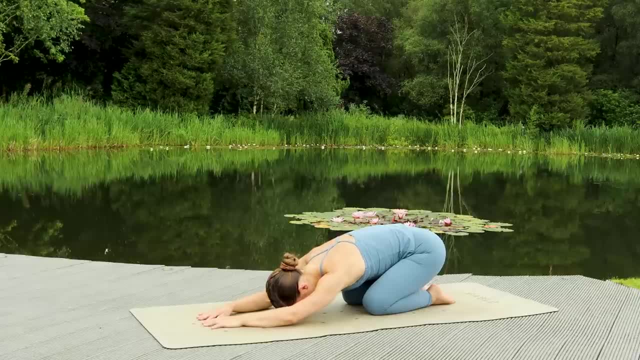 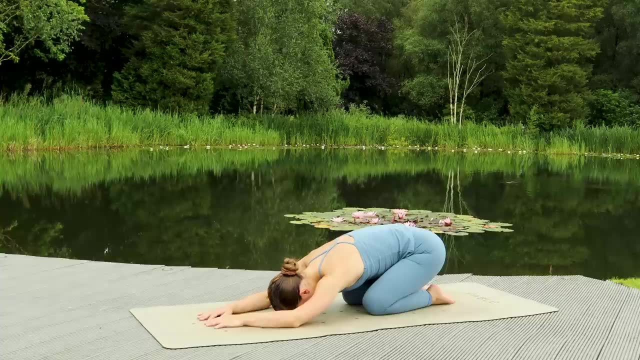 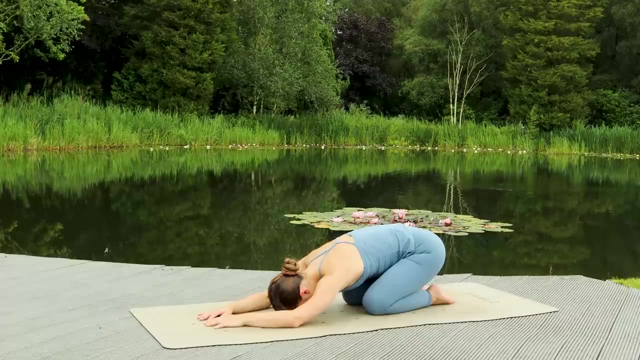 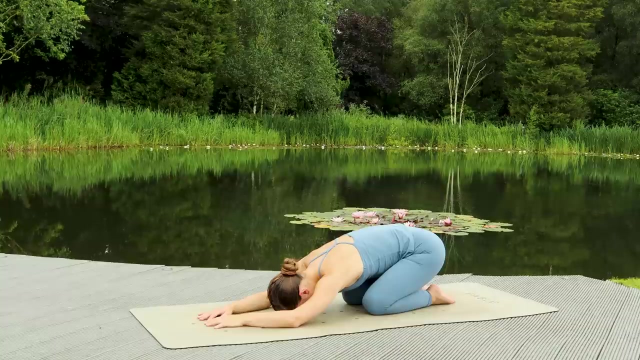 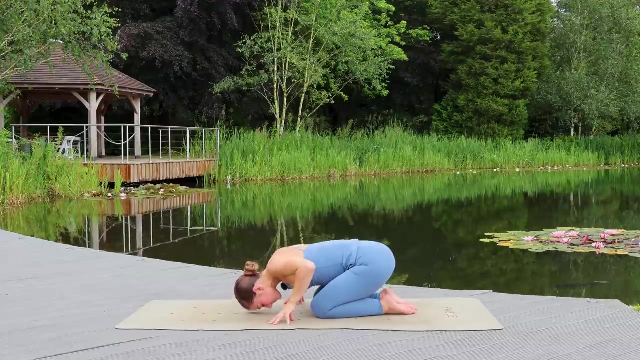 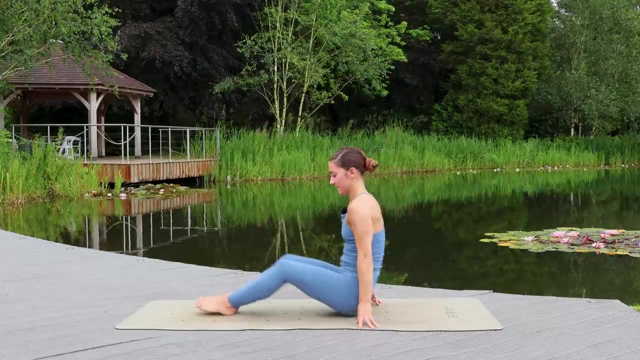 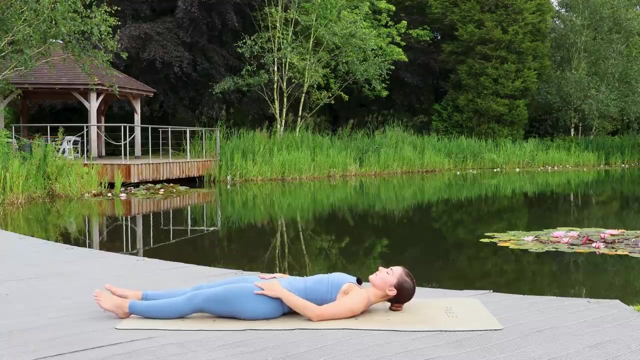 So you can rest your forehead on the mat. Invite your body to relax now And lift yourself up into a kneeling position, Swing your legs around, Come and lie down on your back- Good- And as you lie down, hug your knees into your chest. You're bringing the body into a ball. 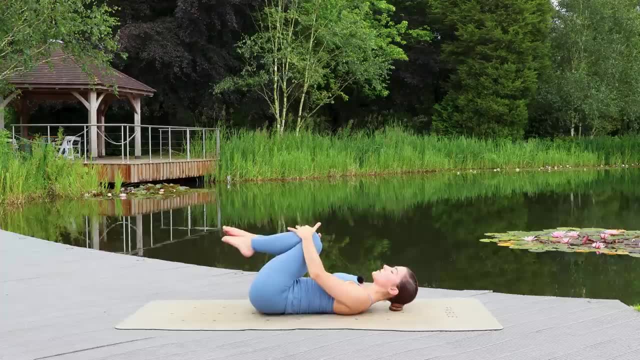 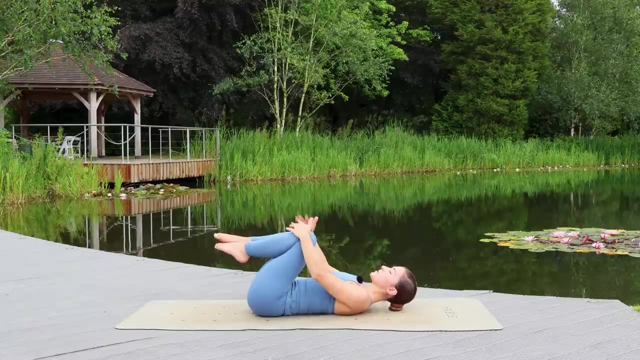 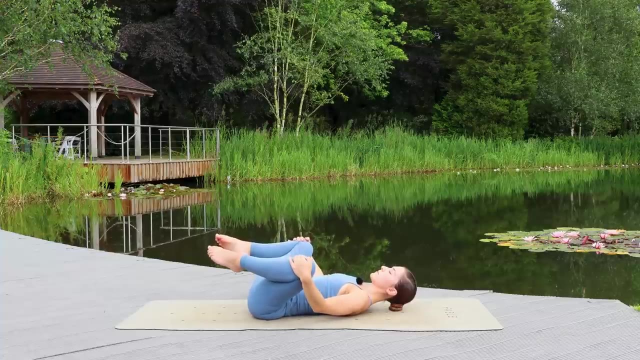 And take a gentle rock side to side, So you're just massaging the back. You have the option to keep the hands on the knees, with the knees together, or you could start to open your knees wide. There's also the option to lift the feet. 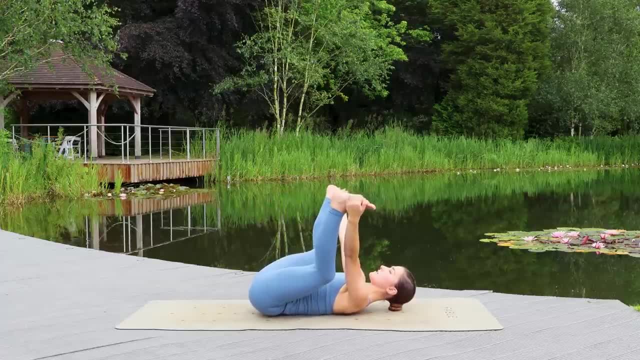 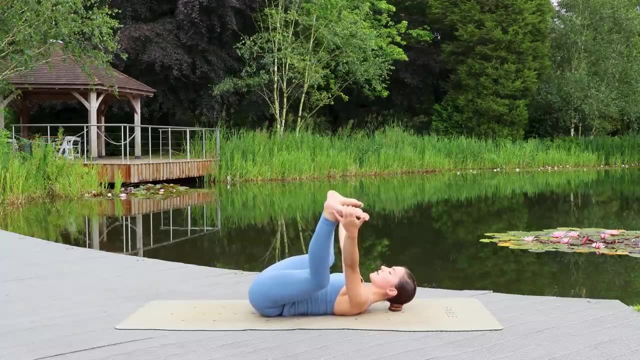 keeping a bend in the knees And as you lie down, hug your knees into your chest But reach the hands to the outsides of the feet for happy baby. And again you could stay in stillness or rock side to side, just finding what feels good. 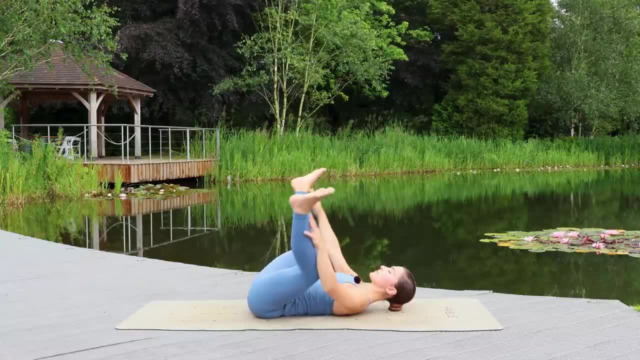 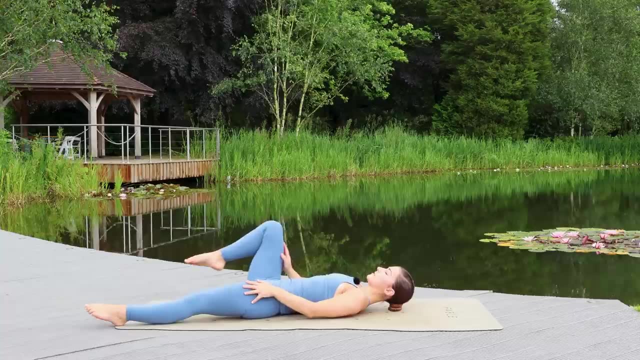 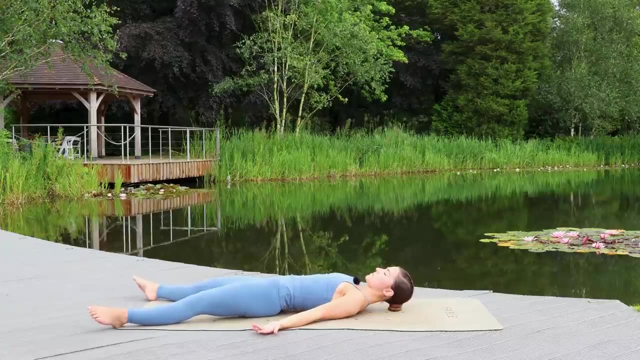 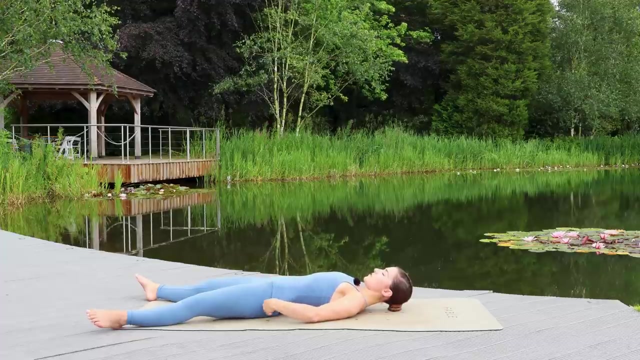 We'll release this position now, One by one. extend your legs down to the mat and relax your arms, either side your body. I find it can help just to take a few moments to fidget, to move in any way you need to before we settle into stillness. Pretty easy, right? So let's take a few moments to manage that stillness. We're going to take a few moments to fidget, to move in any way you need to before we settle into stillness. I'm so excited about that. 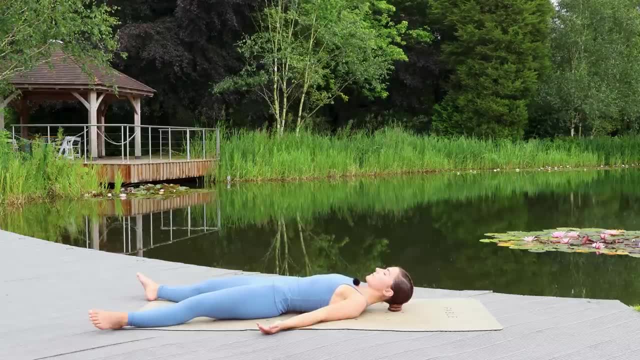 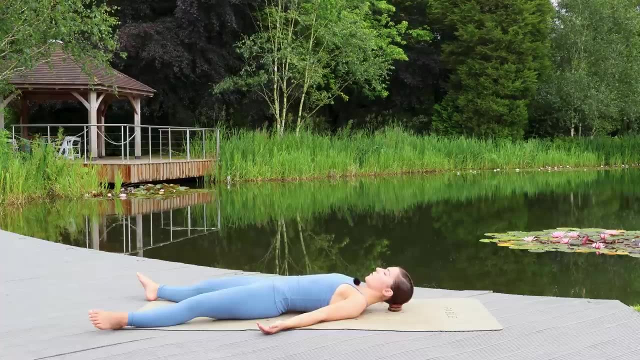 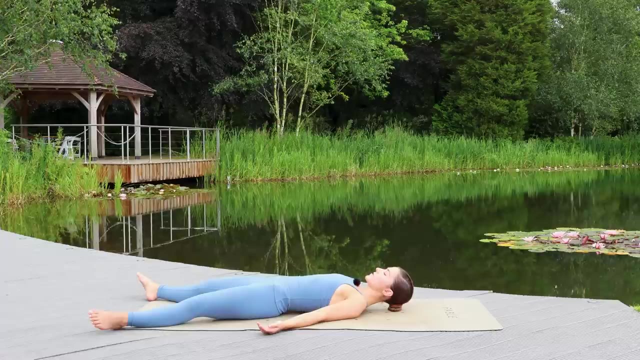 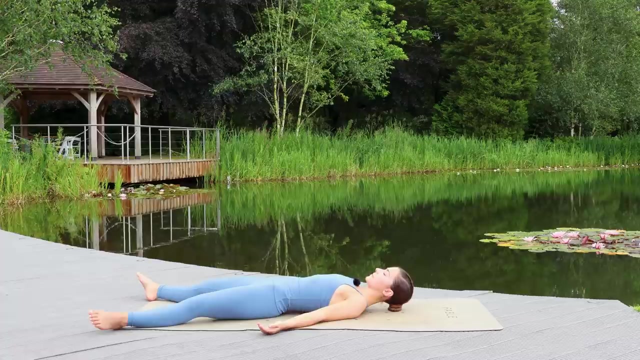 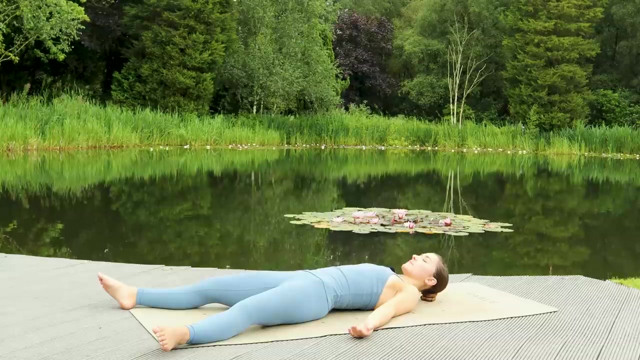 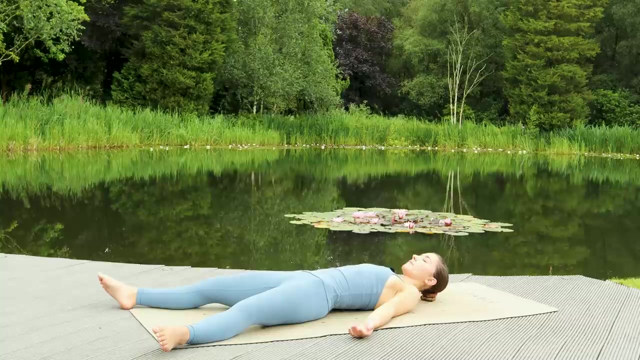 I used to say I love to play this music. I'm so excited about that, and when you're ready, bring all of your awareness back to your breath. let go of any muscular effort as we surrender into Shavasana, Shavasana, Shavasana. 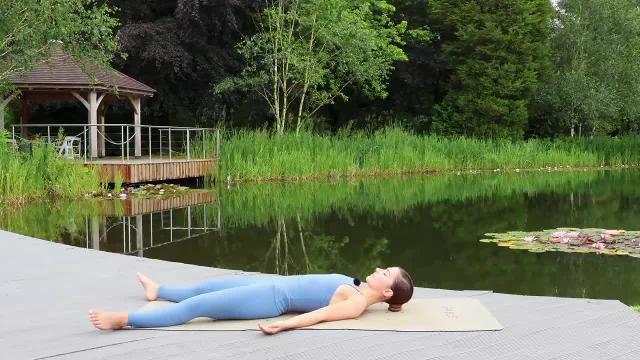 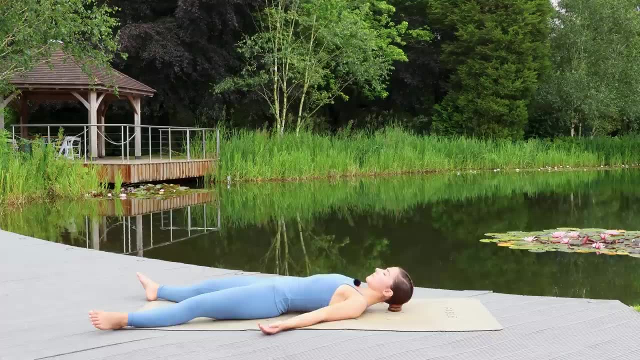 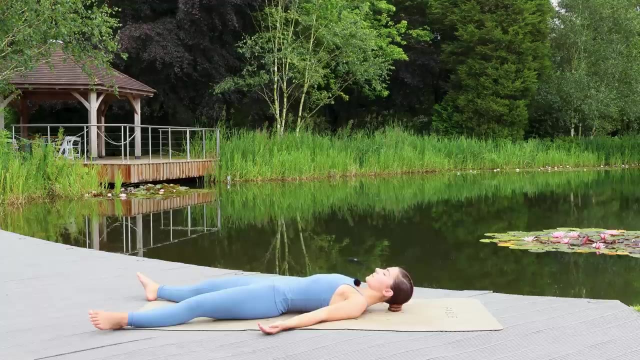 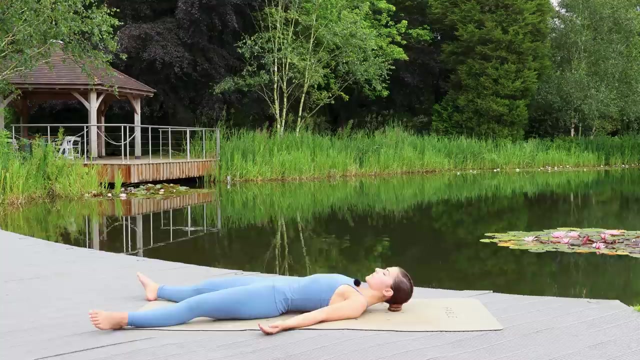 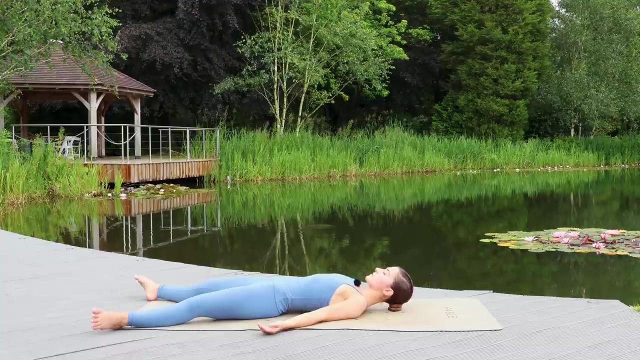 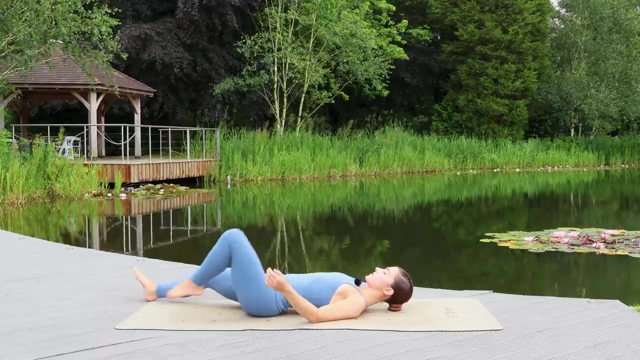 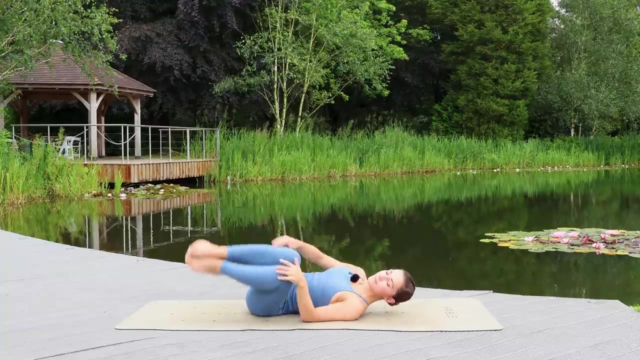 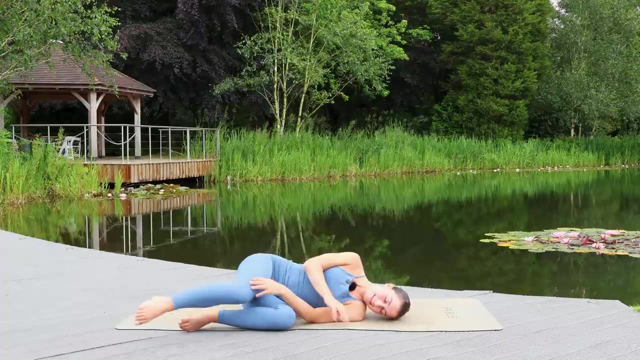 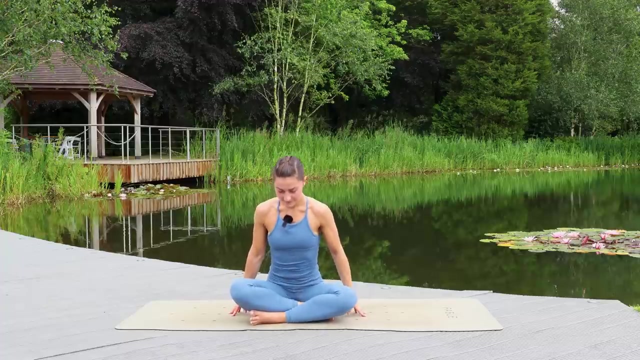 Deepen your breath, bringing your awareness back to my voice. slowly move the fingers and toes, hug your knees into your chest and roll onto your side. when you're ready, join me back in a seated position, just resting your hands on your knees. eyes can stay closed for a moment or two longer.